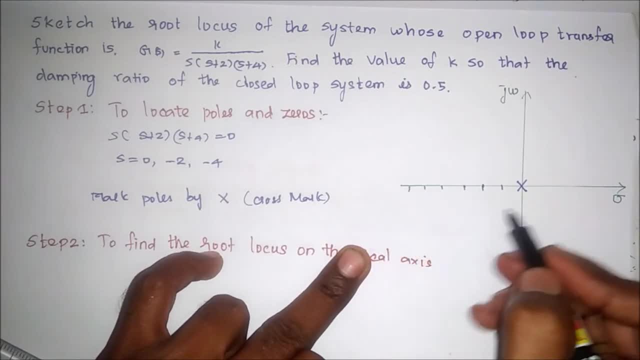 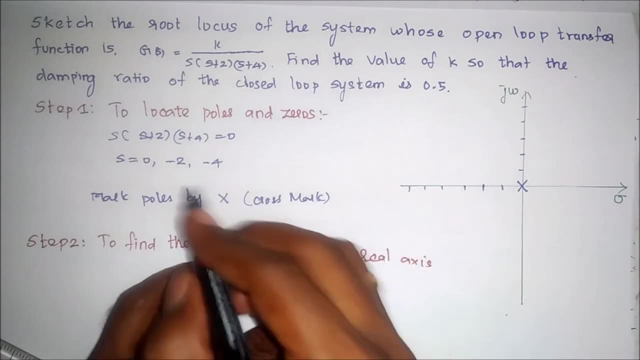 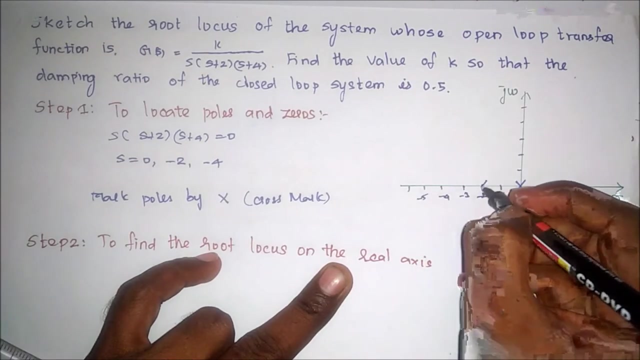 3, 4,, 5, 6.. These are the units in the graph, So now minus 2.. This is minus 1, minus 2, minus 3, minus 4,, minus 5.. Minus 2 is here. Therefore we have to cross mark. 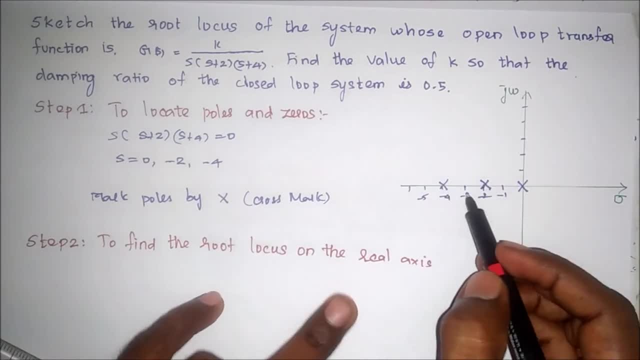 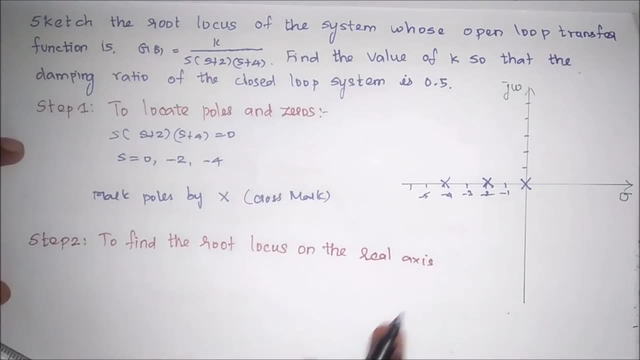 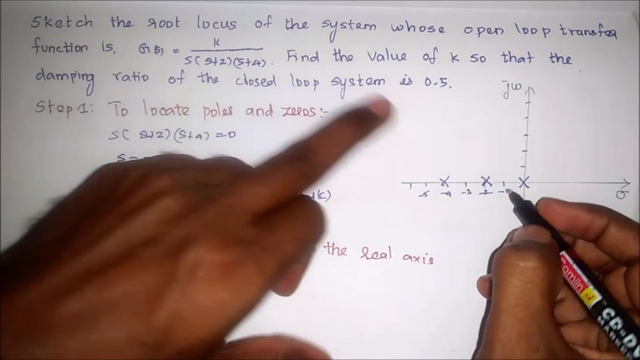 Then minus 4.. So we marked all three poles in the graph. So next, Find the root locus on the real axis. So now, according to the procedure, we have to take a test point. So we can take a test point here. 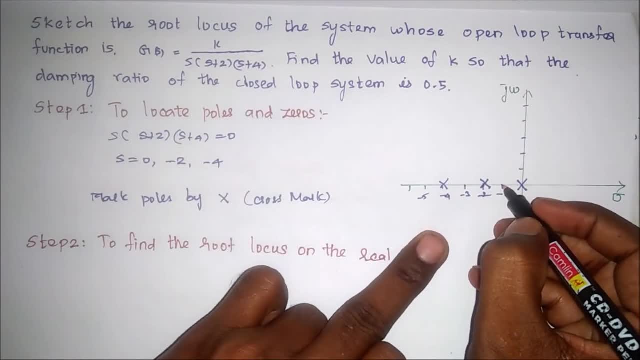 So if we take a test point here based on the concept, from this point right side, there is an odd number of poles and zeros In this problem. there is no zeros, Therefore if the test point is between these two poles. 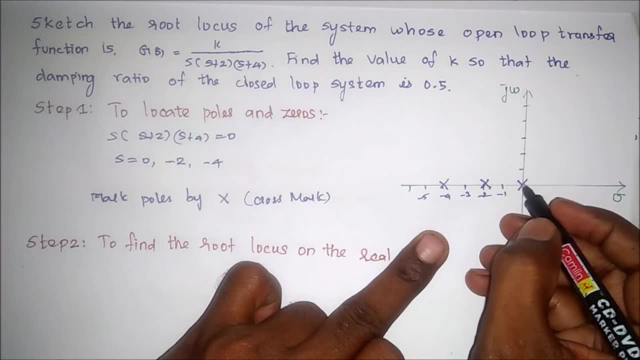 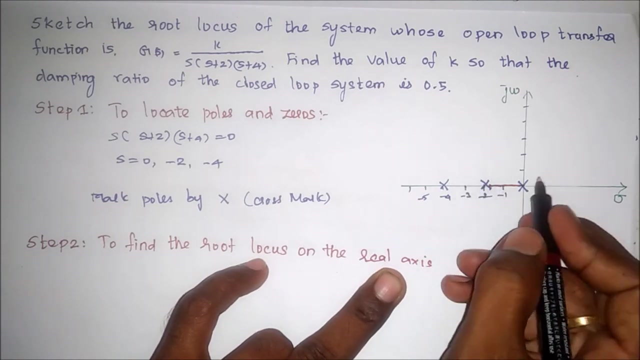 suppose at this point means in the right side there is an odd number of. it means only one pole. Therefore, from this point to this point, definitely root locus. Then if a test point is here means after this point there are even number of poles. 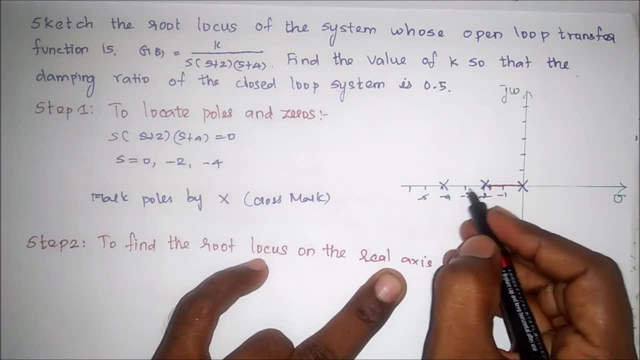 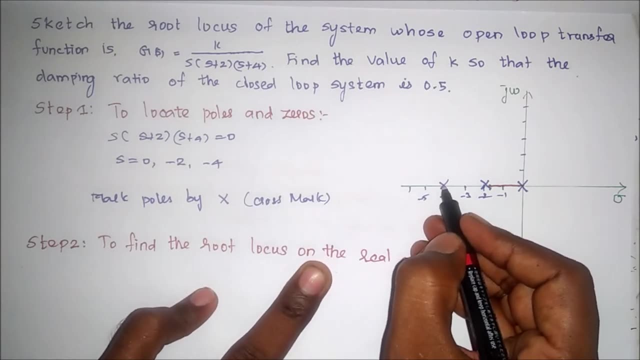 Therefore, from this point to this point it will not be a part of root locus. Then if we take a test point here, it means from this point to infinity in the right hand side of the test point we will be having odd number of poles. 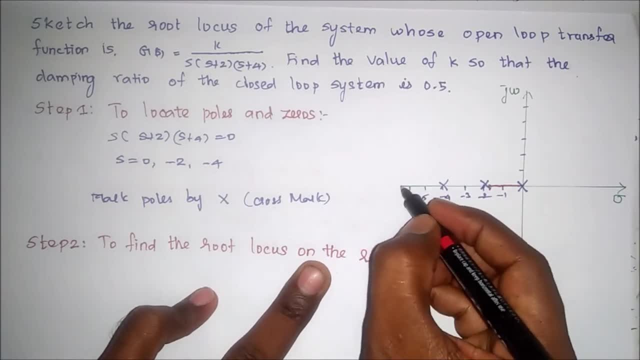 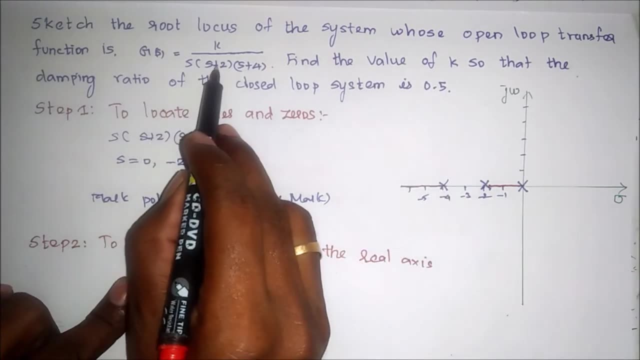 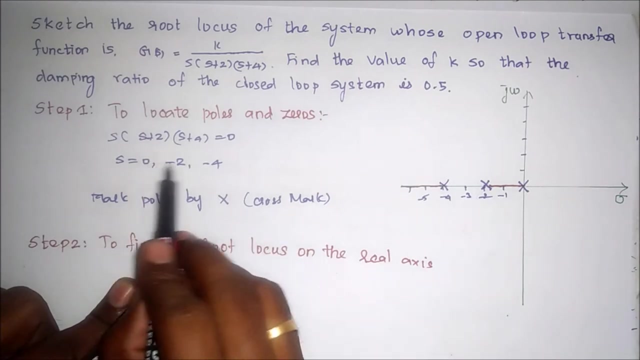 It means three number of poles. Therefore, from this point to infinity, definitely it is a part of root locus. So, according to the concept from the open loop system, the number of poles equal to final number of root locus. Here there are three number of poles. 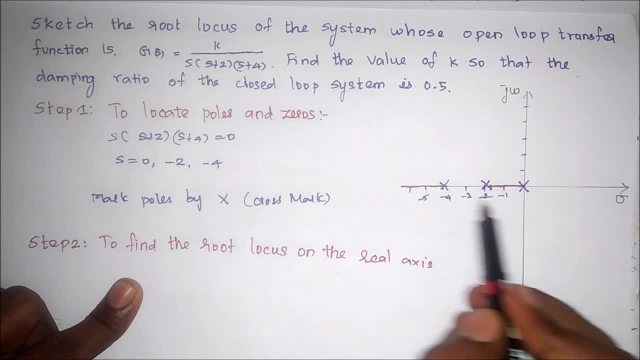 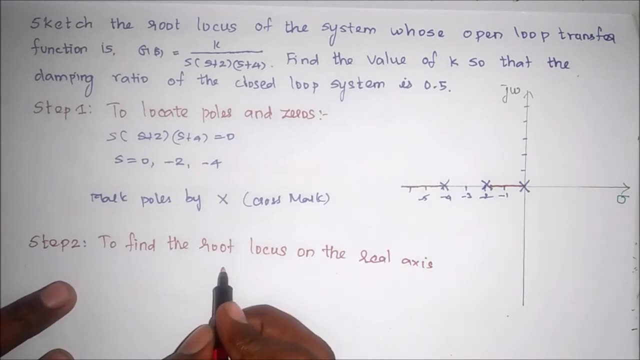 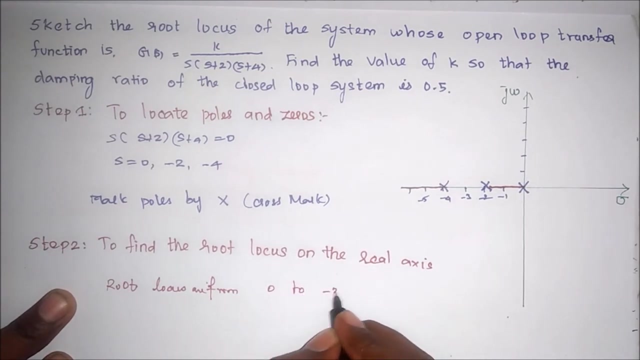 Therefore three root locus will be available Here. so far there are two root locus, But we have to find the third root locus, So here we have to write root locus, Or from 0 pole to minus 2 pole and minus 4 pole to infinity. 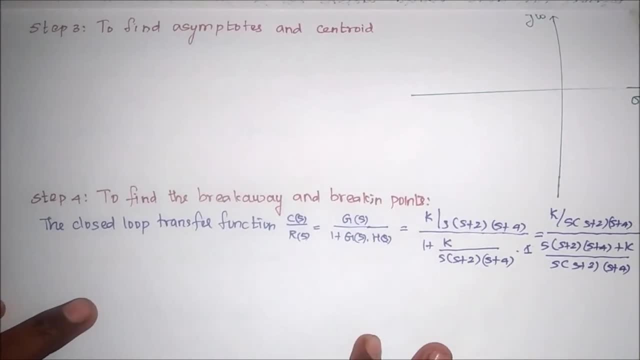 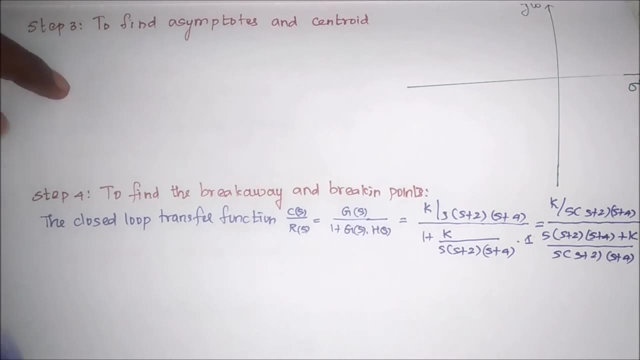 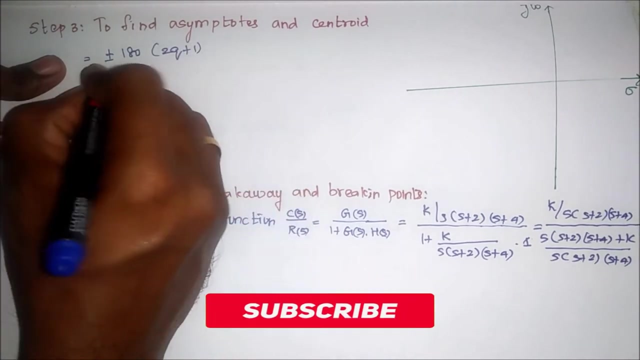 Next we have to find the angle of asymptotes and centroid. So we know the formula Usual to calculate the angle of asymptote is angle of asymptote equal to plus or minus 180.. So angle of asymptote equal to plus or minus 180 divided by 2Q plus 1, divided by number of poles minus 0s. 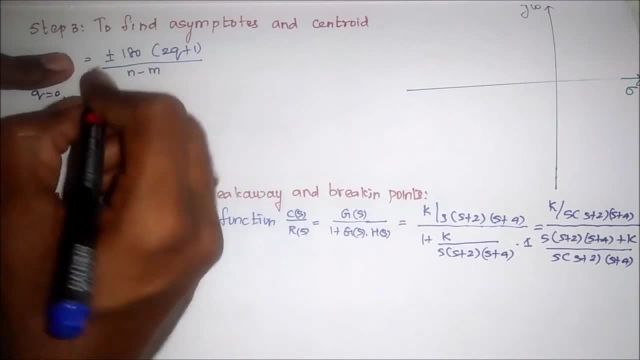 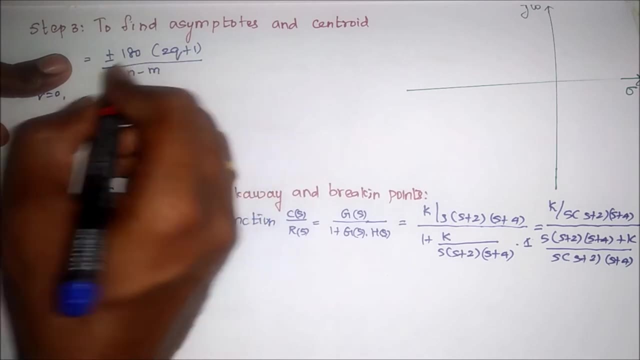 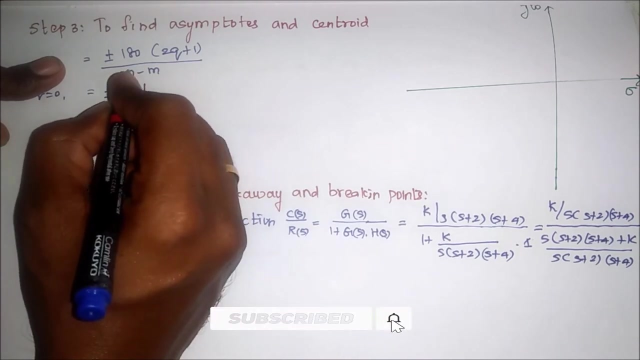 So now if Q equal to 0. So now we have to substitute Q equal to 0. Then 0 into anything 0 plus 1, 180.. Therefore plus or minus 180 divided by here in the given problem, number of poles 3.. 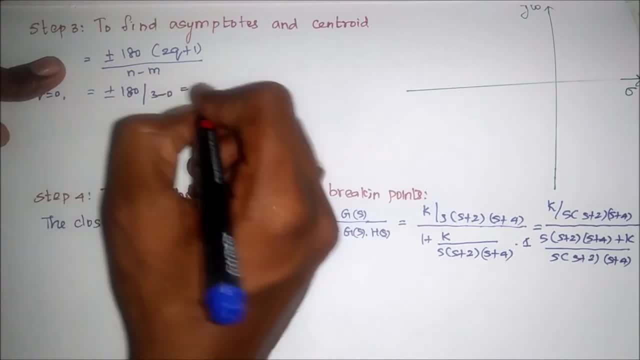 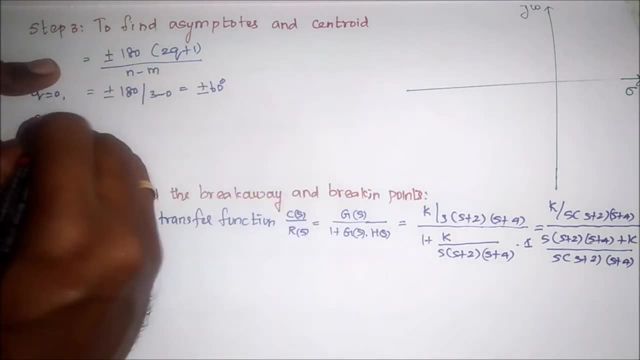 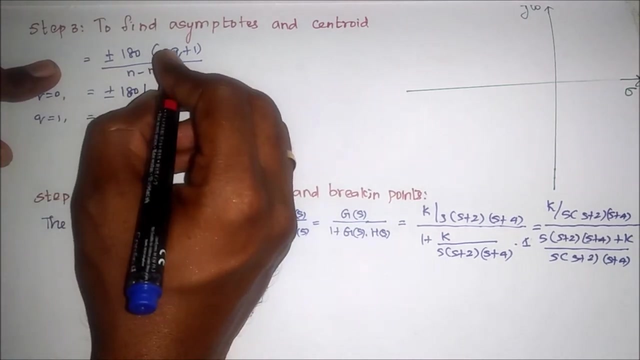 Number of 0s, 0. So angle of Asymptote equal to plus or minus 60 degree. Suppose Q equal to 1, we have to substitute. We will get plus or minus 180 into 1.. 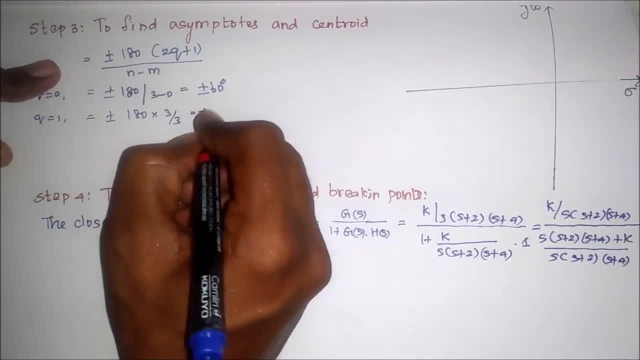 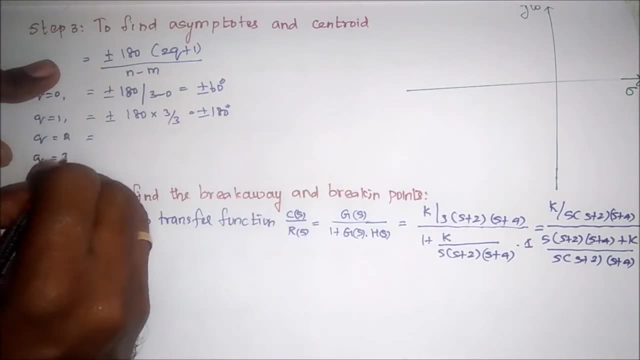 So 2 plus 1, 3 divided by 3.. So we will get plus or minus 180 degree. So now Q equal to 2, we have to substitute Similarly, Q equal to 3, we have to substitute. 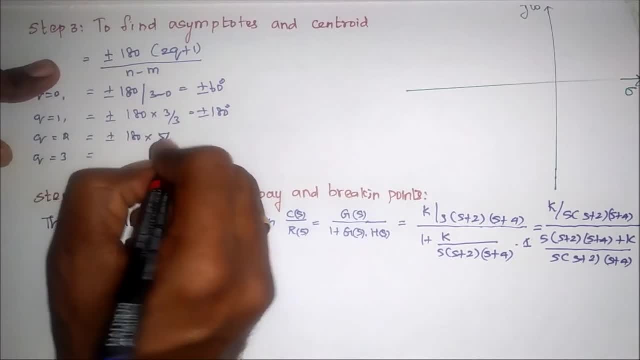 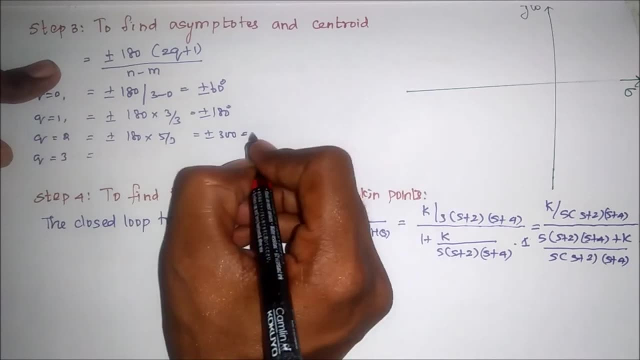 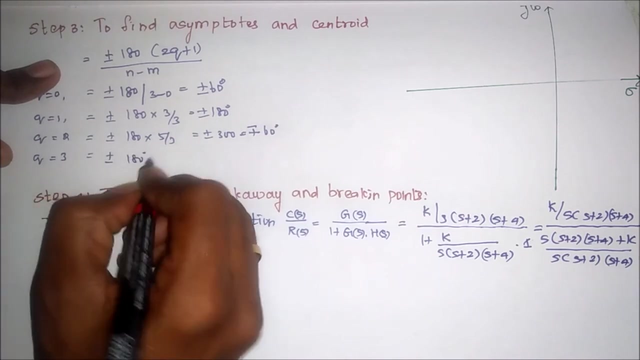 We will get 180 into 5 divided by 3. Equal to plus or minus 300.. So it is almost equal to minus, to plus 60 degree. Then Q equal to 3, if we substitute, it will come 180 into 7 divided by 3.. 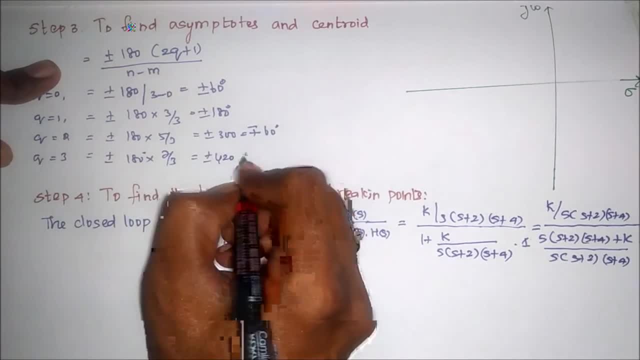 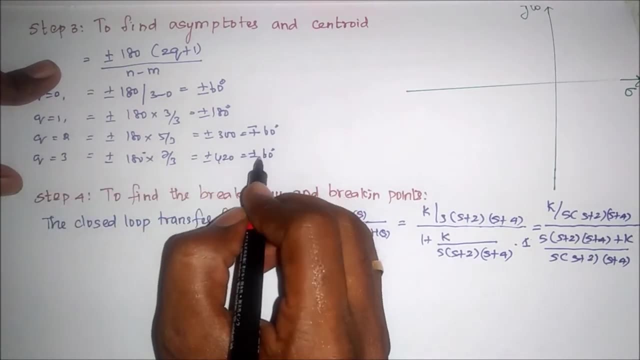 So now it will be 420.. So it is equal to plus or minus 60 degree. So almost. if we substitute Q values further, its value will be definitely plus or minus 60 only. So angle of asymptote is the first finite angle. 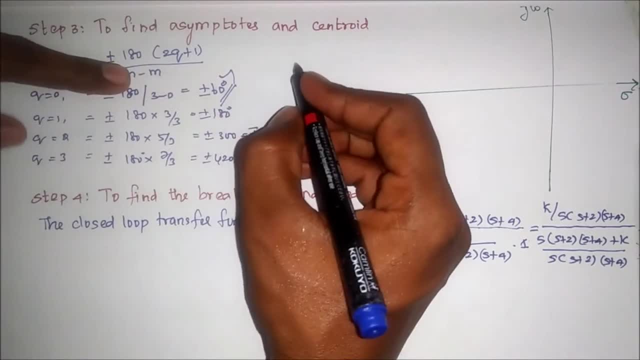 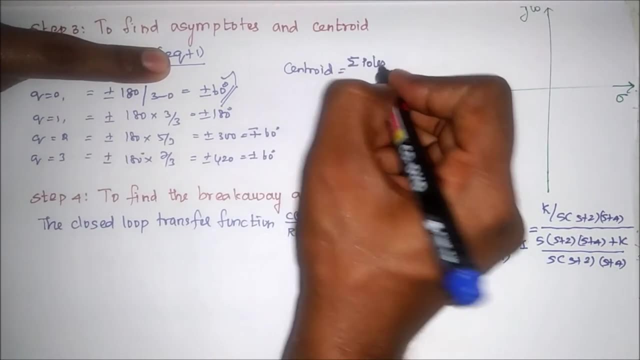 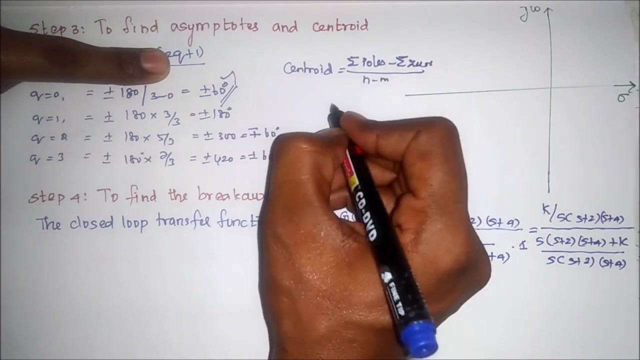 So this is The angle of asymptote. Next centroid: Centroid. To calculate the centroid, the formula is: sum of poles minus sum of zeros divided by number of poles minus 0. Therefore, sum of poles: Poles equal to 0. 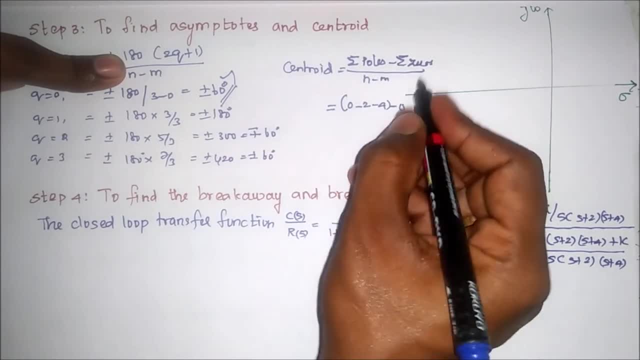 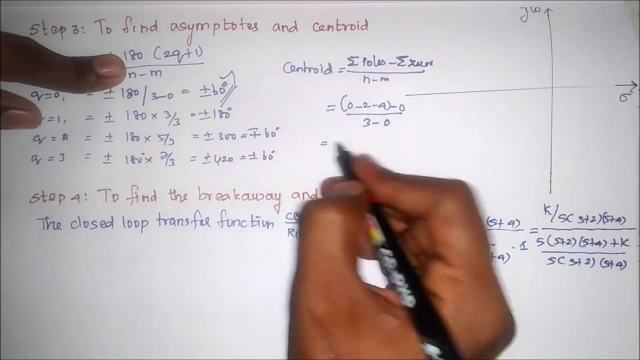 Then minus 2, minus 4, minus, There is no 0 in this problem. Therefore, 0 divided by 3, number of poles, Minus minus 0, number of zeros. Therefore, minus 6 divided by 3, equal to minus 2.. 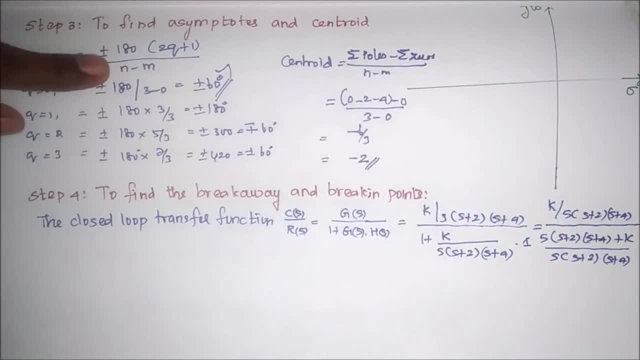 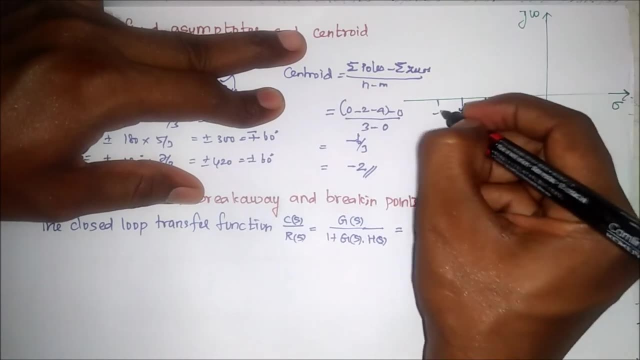 Minus 2 is the centroid. Therefore in the graph suppose this is minus 1, minus 2, minus 3,, minus 4, minus 5.. Means here: minus 2 is the centroid. So this point is the centroid. 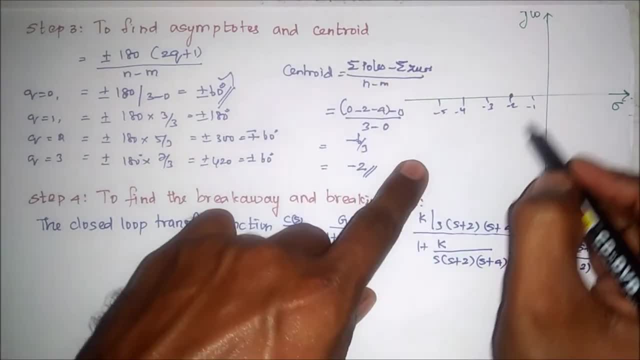 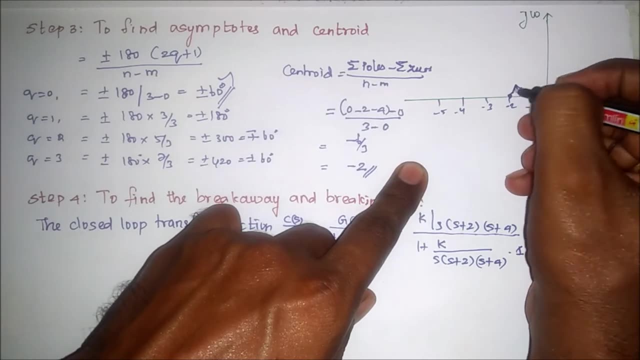 From this angle is plus or minus 60 degree From this real axis. so we have to take 60 degree angle exactly. Then we have to, By using dot-dot line, we have to mark like this: Then similarly, minus 60 degree. 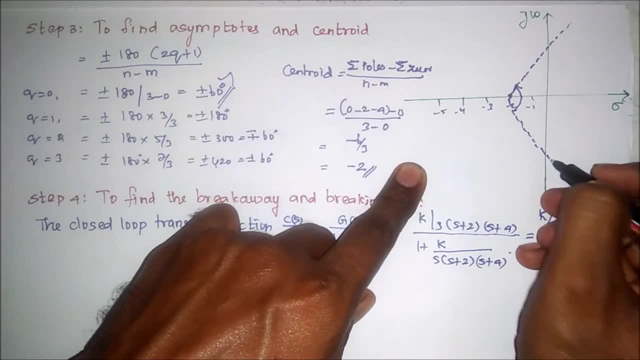 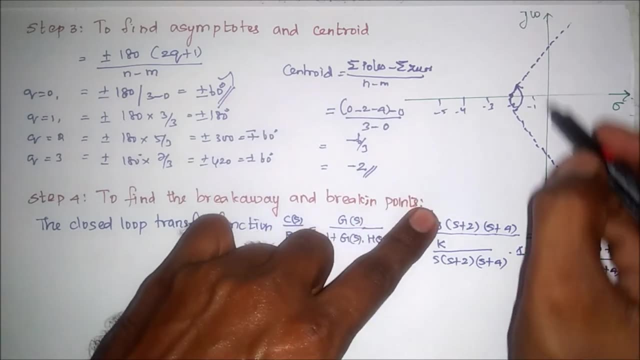 it will come in the bottom side. So by using scale and projector we have to exactly mark 60 degree. Then we have to draw the dot-dot line. So this is the asymptotes. Its centroid is minus 2.. 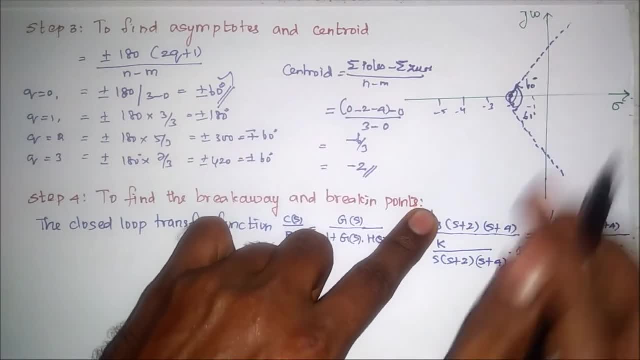 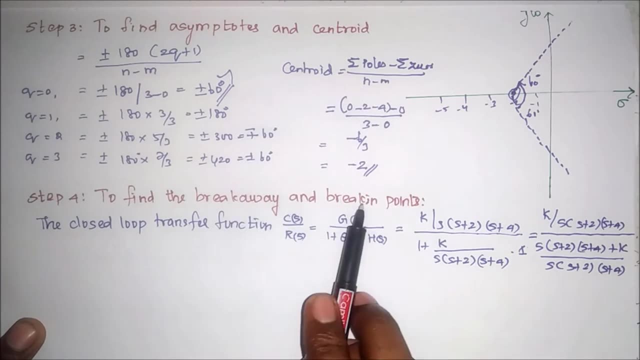 Angle of asymptotes are plus 60, minus 60.. Next, to find the break-away and break-in points. Actually, to find the break-away and break-in points, we have to know the characteristics equation. Actually, in the given problem, 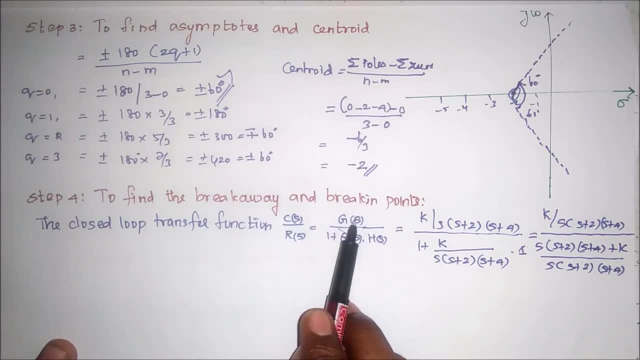 we have been given the open-loop transfer function G. To get the characteristic equation we have to find the closed-loop transfer function. The formula to calculate closed-loop transfer function from open-loop transfer function is G divided by 1 plus G. So from the given problem. 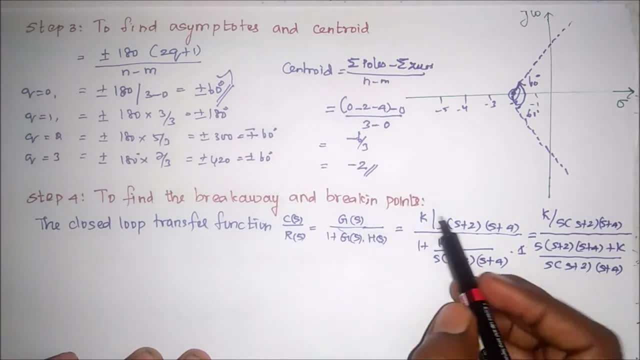 we can assume H equal to 1.. So now G equal to K divided by S into S plus 2, into S plus 4, divided by 1 plus G, equal to K, divided by S into S plus 2, into S plus 4.. 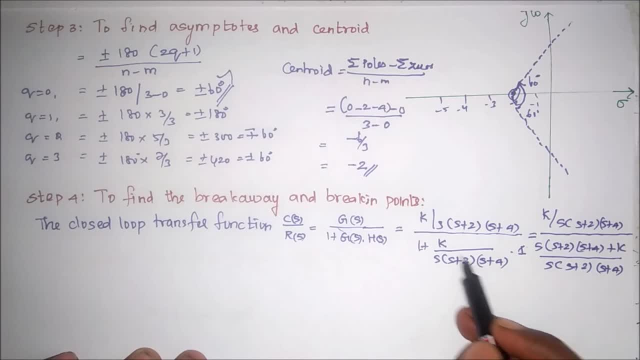 Here gain we considered as unity, Then we have to take LCM. So if we take LCM we will get this equation. So here this term and this terms are same. Therefore, finally, K transfer function equal to: 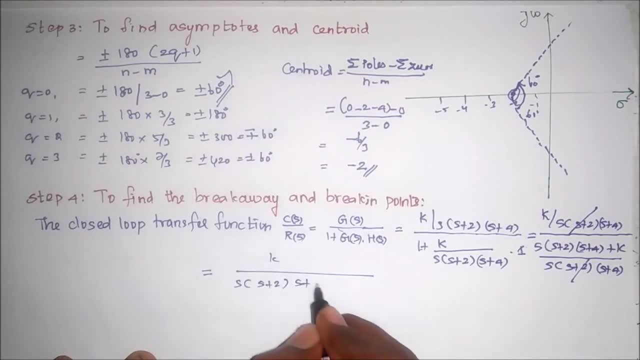 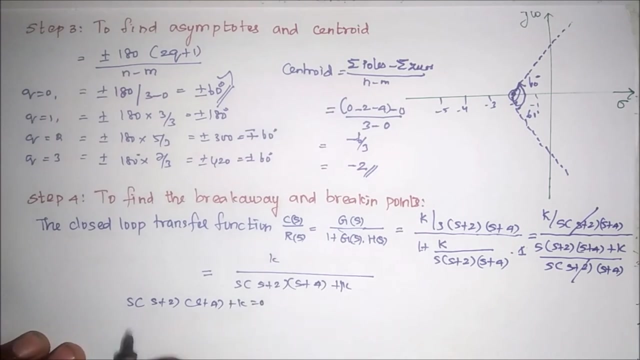 K divided by S into S plus 2, into S plus 4 plus K. So now, this is the characteristics equation. So now characteristic equation is S into S plus 2, into S plus 4 plus K, equal to 0.. 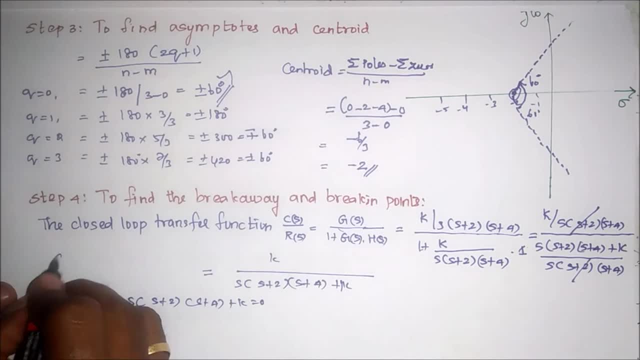 To find the break-away or break-in point. the condition is: TK divided by DS equal to 0.. By using this condition, we have to find the roots, Then we have to find the K. Based on the K value, we can know whether the given problem is having break-away point and break-in points. 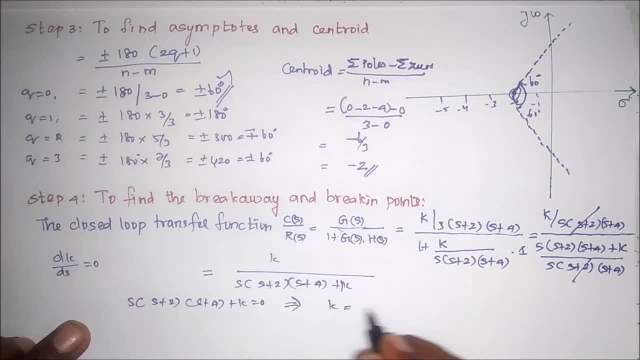 So now, from this K equal to minus S into S plus 2, into S plus 4.. So now we have to multiply all these three terms. So now, if we multiply these two, we will get S into S square plus 6S plus 8.. 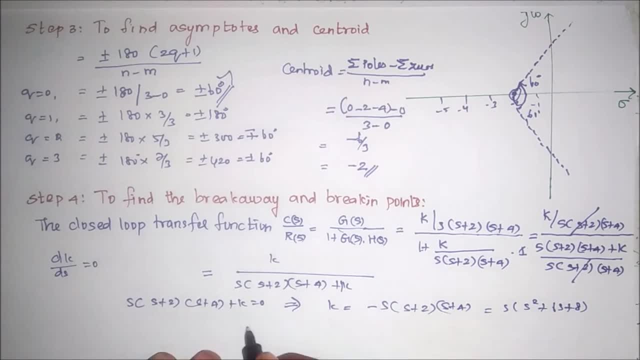 So again we have to multiply S inside, So we will get S cube plus 6S square plus 8S. So this is the K value. So now we have to find DK with respect to S. So now this will be 3S square. 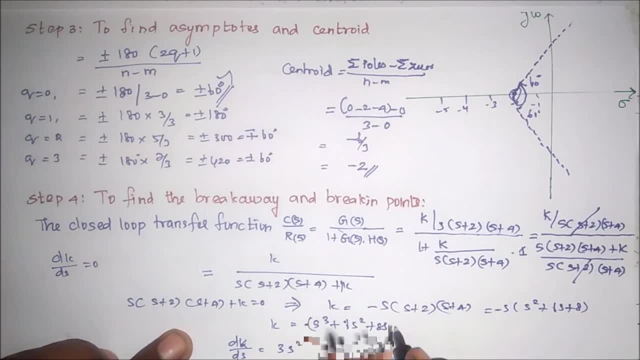 Here minus, Therefore here also minus will come. So minus 3S square plus 12S plus 8, equal to 0.. Therefore, from this 3S square plus 12S plus 8, equal to 0.. 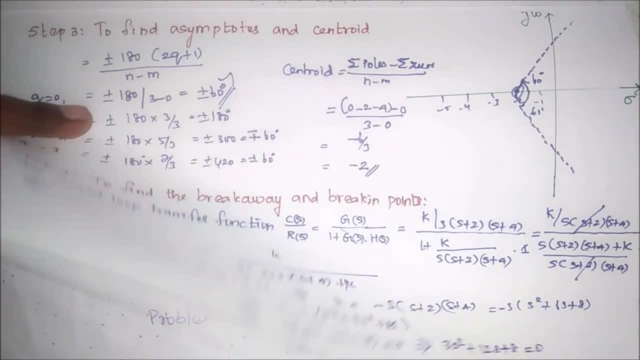 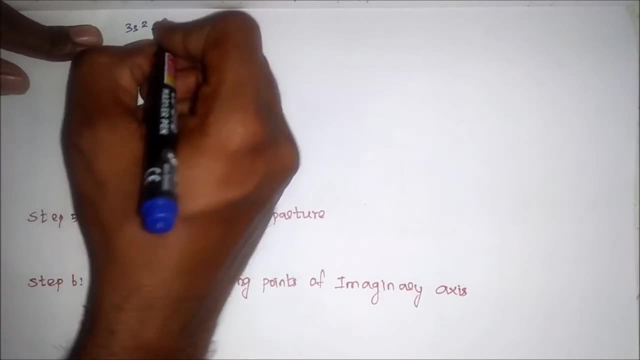 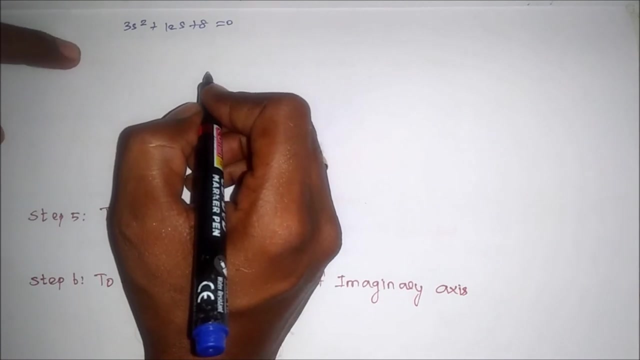 So for this equation we have to find the roots Now. so we got this quadratic equation: 3S square plus 12S plus 8, equal to 0.. From this, so we know the formula to find the roots. 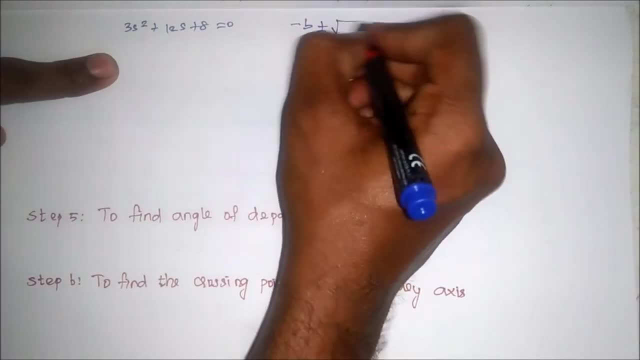 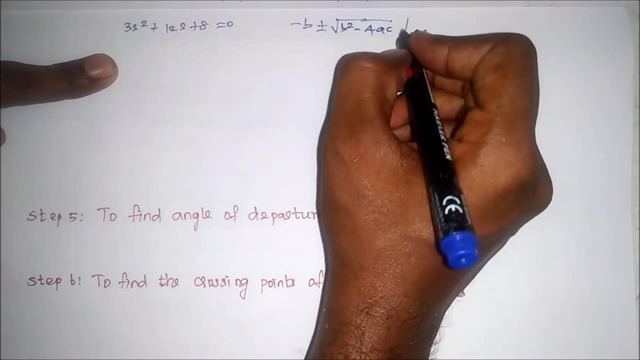 So we know: minus B, plus or minus square root of B, Square root of B square minus 4AC divided by 2A. This is the formula to find the roots for a quadratic equation. So here A is 3.. B is 12.. 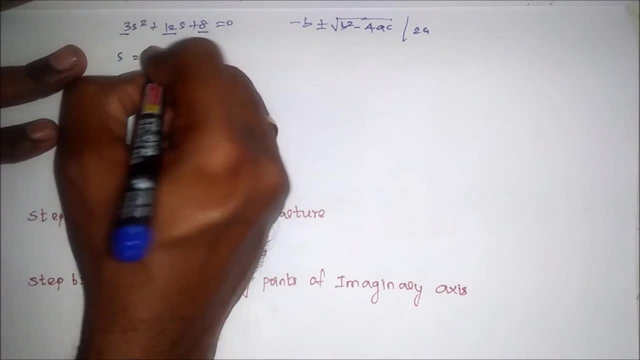 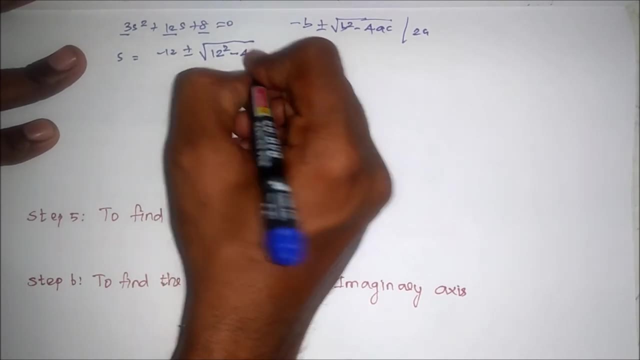 C is 8.. Therefore, roots S equal to minus, B minus 12, plus or minus square root of B, square minus 4A equal to 3.. C equal to 8.. 4AC divided by 2A, 2 into A is 3.. 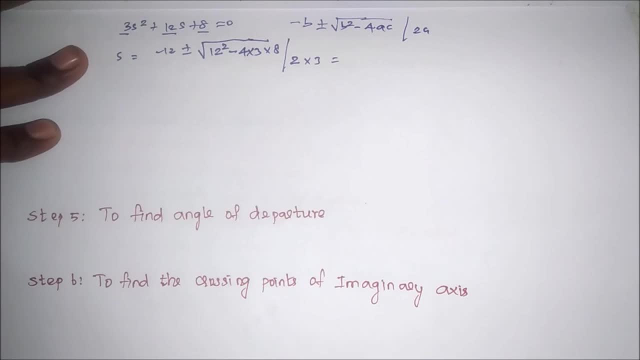 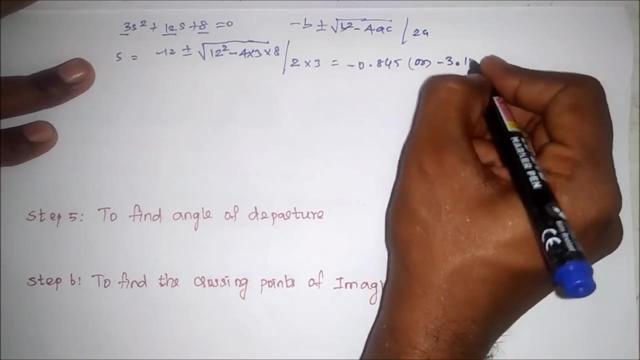 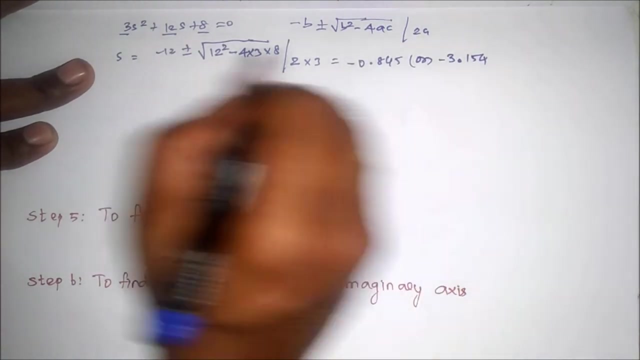 So now we will get minus 0.845 or minus 3.154.. So after solving this term we will get minus 0.845, or because here we are having plus or minus, Therefore here minus 12.. Here some value will come. 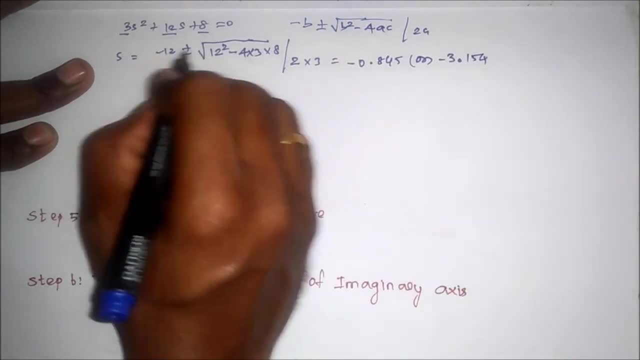 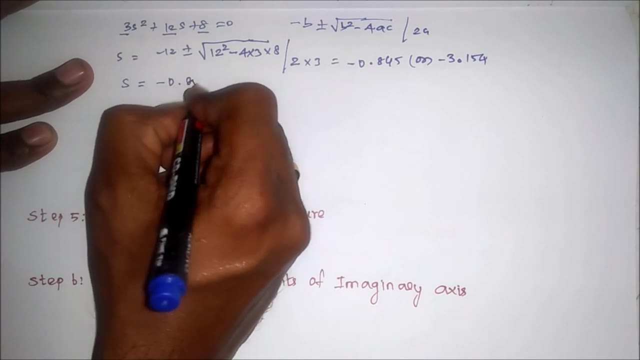 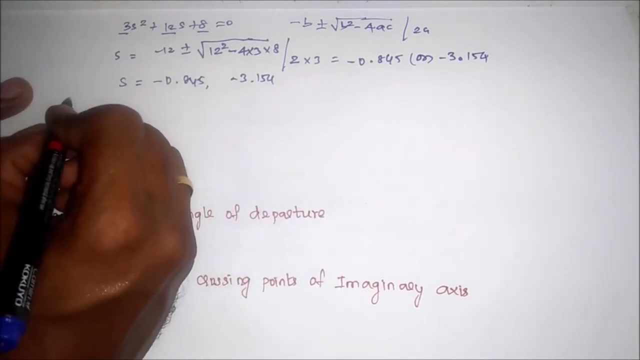 So first we have to use plus, Then we will get this answer, Then we have to use minus, We will get this answer. So now roots are S equal to minus 0.85.. Then minus 3.154.. So now we have to substitute first S1 value. 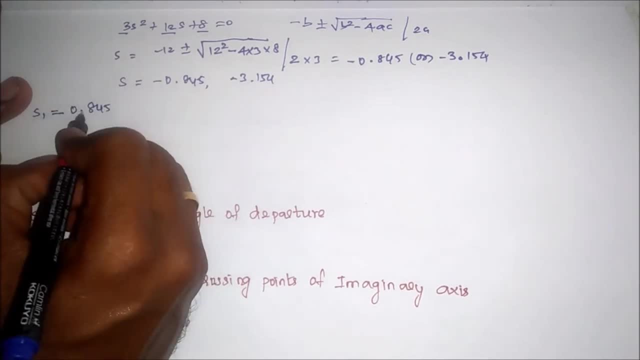 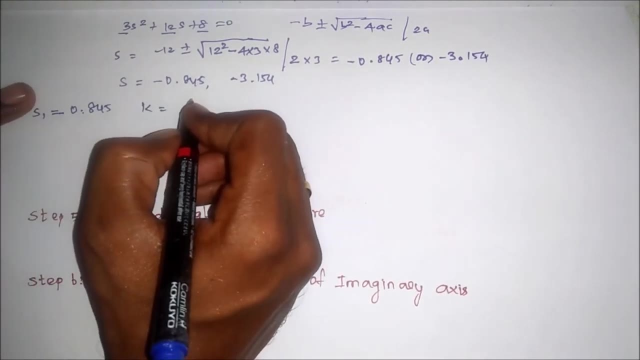 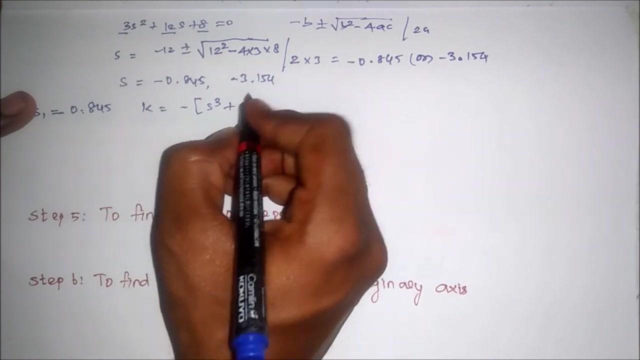 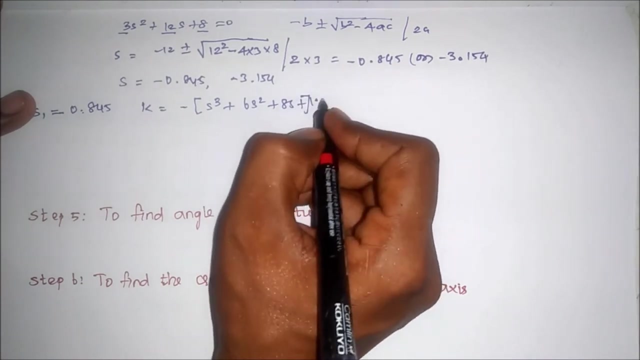 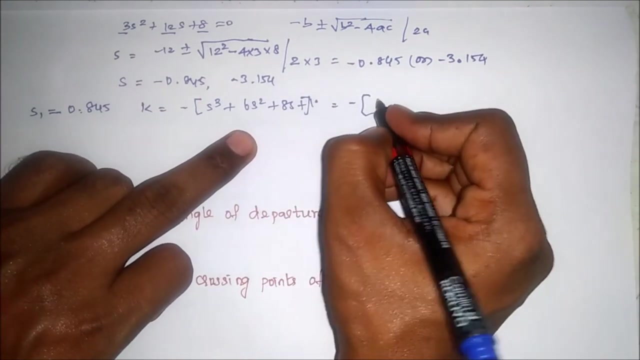 Minus 0.854 into K equation, K equal to. So we know K equal to minus Minus S, cube plus 6S, square plus 8S. So now we have to substitute this S1 value, So here, minus of minus 0.845, the whole cube. 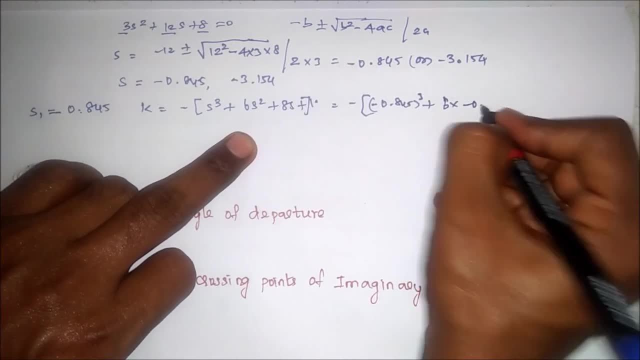 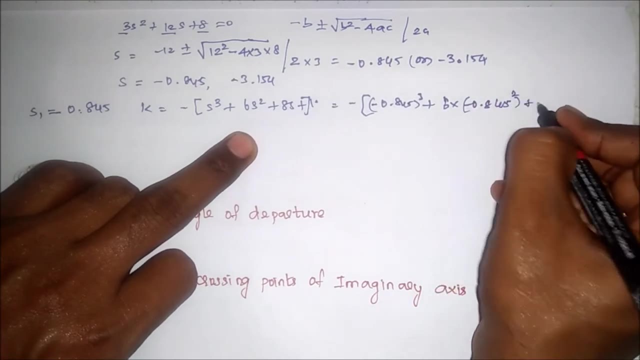 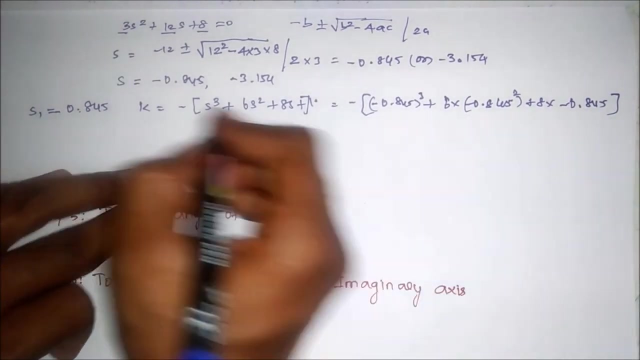 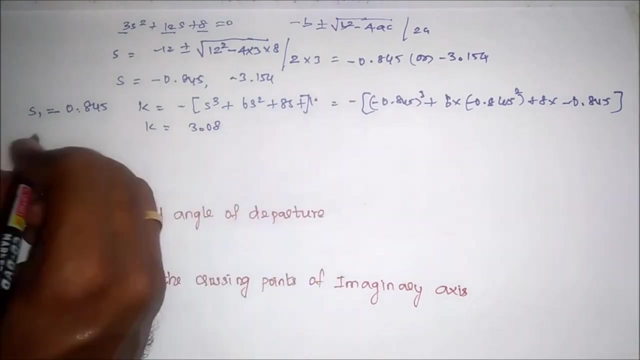 Plus 6 into minus 0.845.. The whole square, plus 8 into minus 0.845.. So now from this we will get K value equal to 3.08.. So now we will substitute S equal to minus 3.154.. 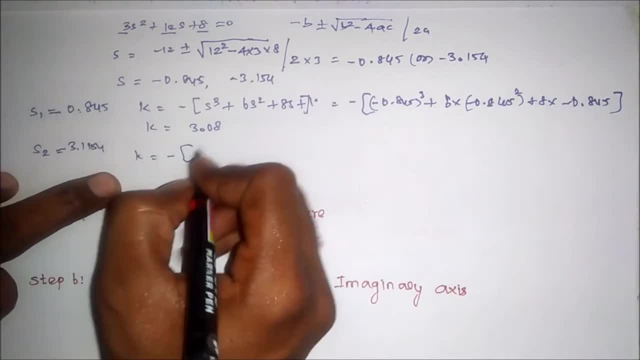 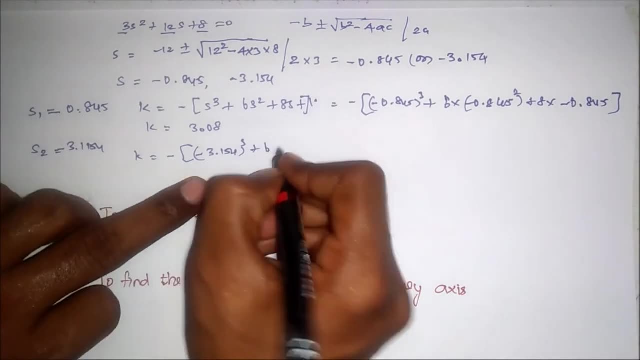 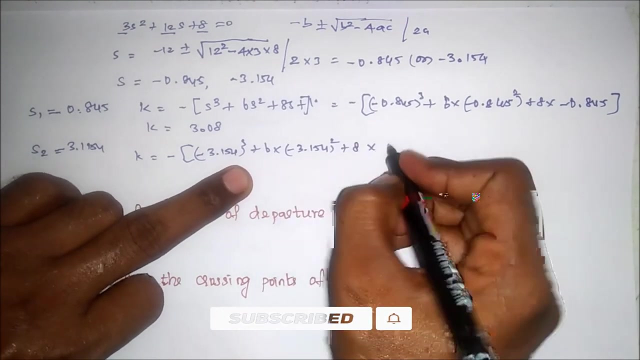 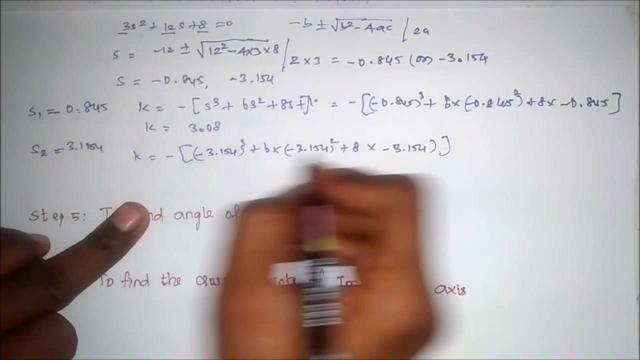 So now K equal to minus of minus 3.154.. The whole cube plus 6 into minus 3.154.. The whole square plus 8 into minus 3.154.. So now K equal to minus 3.05.. 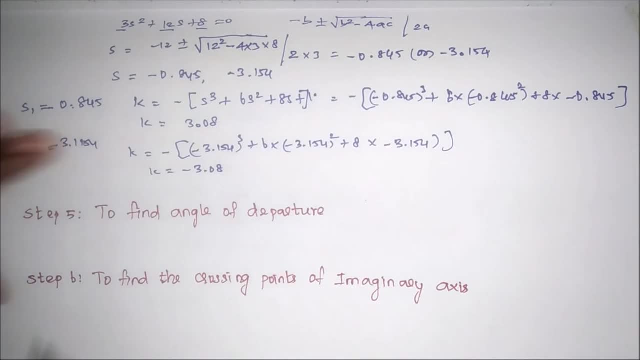 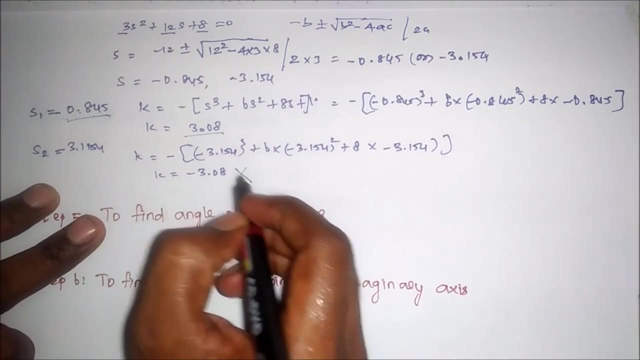 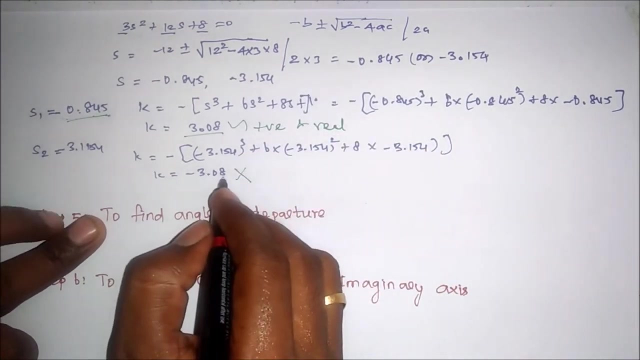 So from this we see, for this root K is positive, But for this root K is negative, So it is a positive and also real value. This is not a positive, negative value. Therefore this point is a break away point. 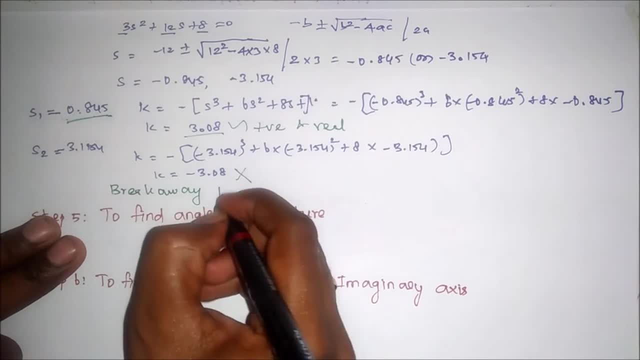 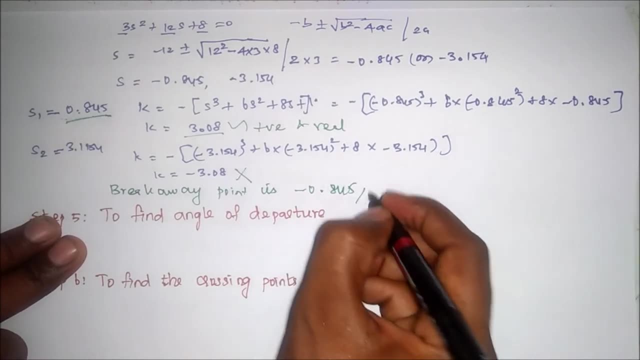 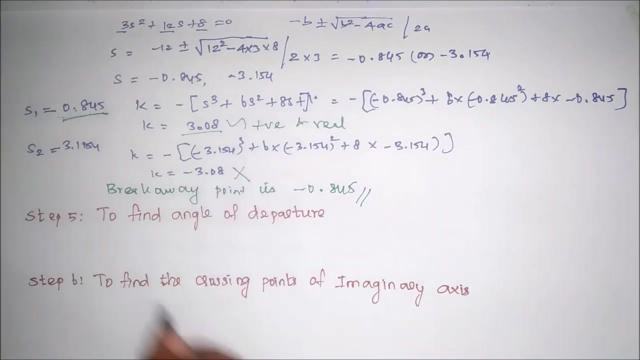 Break away point is minus 0.845.. This is the break away point. But this point is not break away point because it is negative value. So now we have to find the angle of departure. So formula to calculate the angle of departure is: 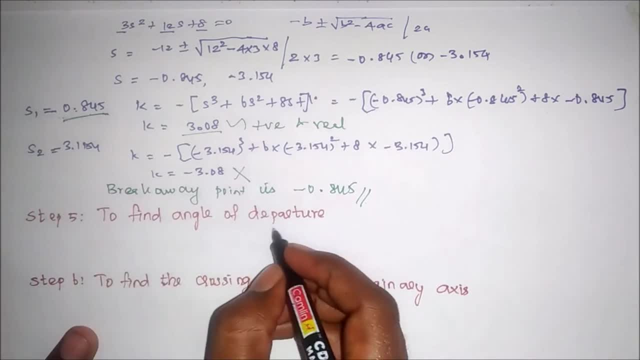 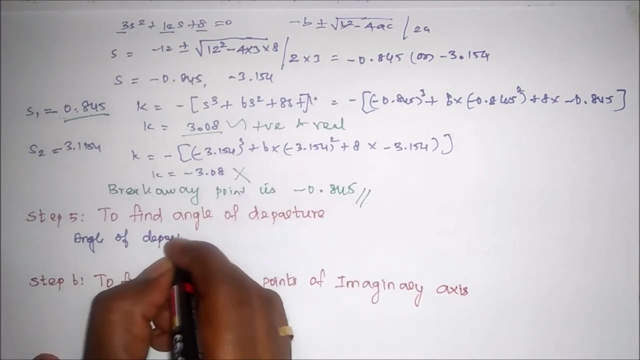 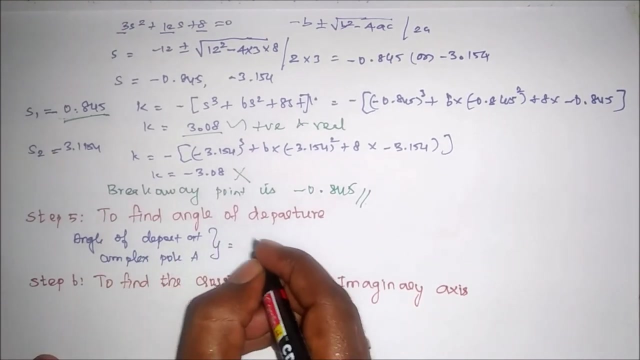 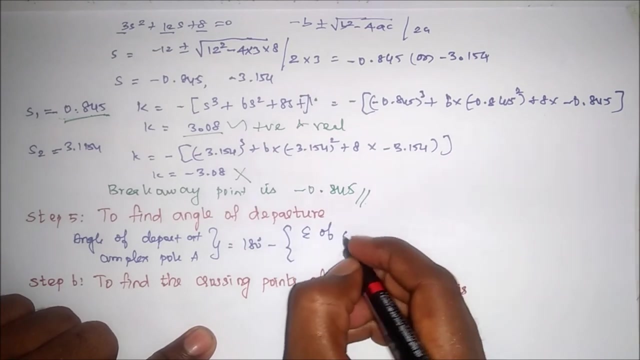 So if we have complex pole, we can calculate the angle of departure. Or if complex pole is available in the given problem, angle of departure will be there, Because the formula for calculating angle of departure is angle of departure at complex pole, A equal to 180 minus sum of angles of poles from complex pole. 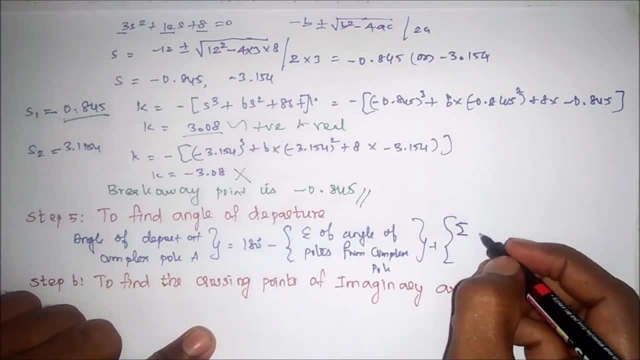 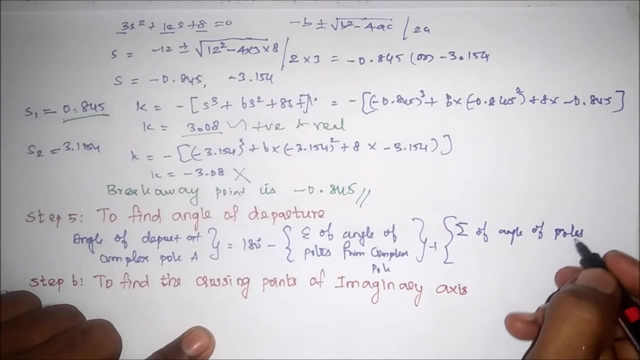 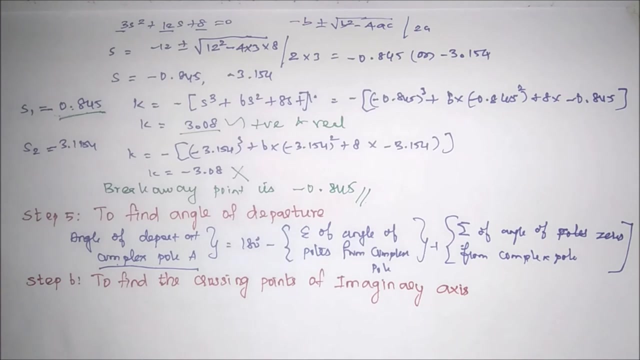 Plus sum of angles of poles, Sum of angles of zeros from complex pole. We do not have complex pole in this problem. Therefore here there is no angle of departure. There is no angle of departure, So next we have to find the crossing point of imaginary axis. 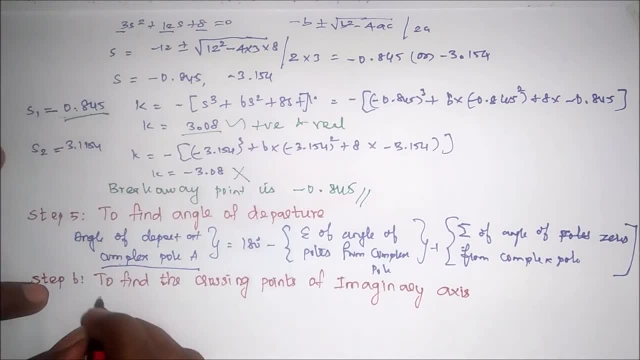 So from the characteristic equation We know. characteristic equation is s cube plus 6s, square plus 8s plus k, equal to 0.. So now we have to substitute: Let s equal to j omega. We have to substitute into this equation. 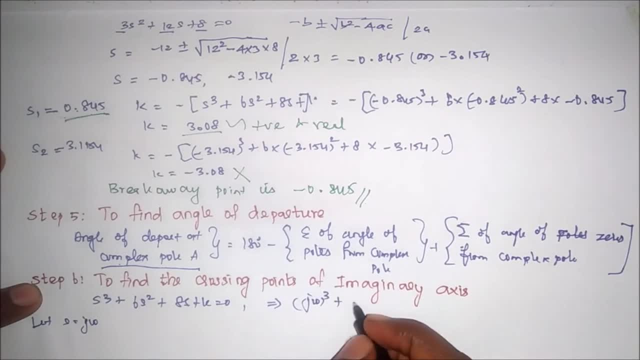 So now j omega cube plus 6 into j omega square, plus 8 into j omega plus k, equal to 0.. So now, from this minus j omega cube, So from this minus 6 omega square, From this plus 8 j omega plus k equal to. 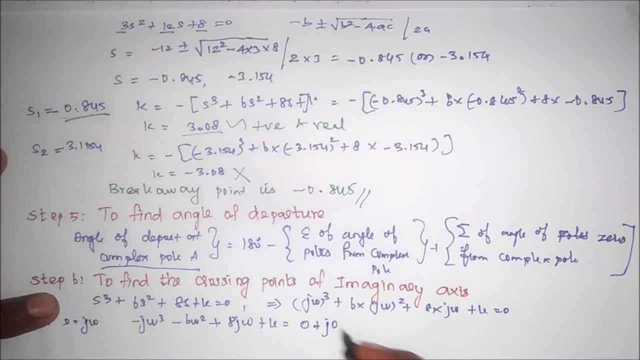 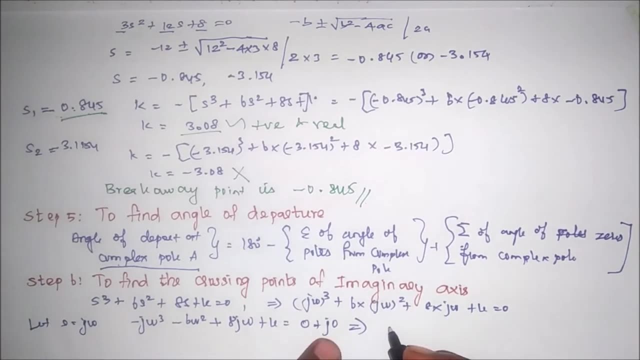 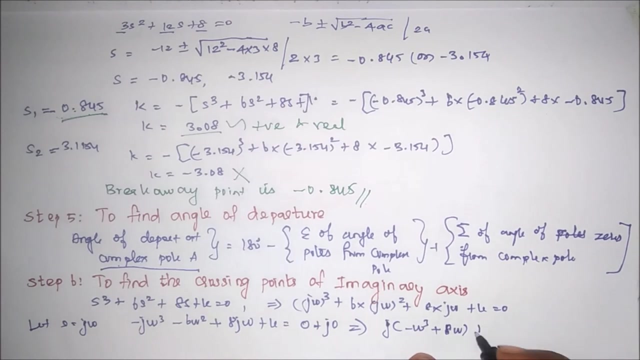 So we can write this: 0 as 0 minus 0 plus j 0.. So now we can separate this into real and imaginary part. So from this, So we can separate imaginary part alone. So, minus omega 3 plus 8 omega minus 6 omega square plus k, equal to 0 plus j 0.. 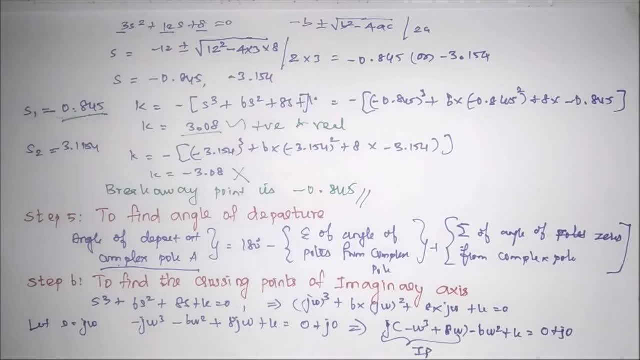 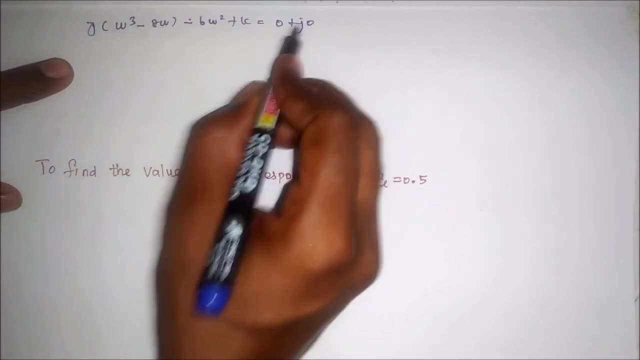 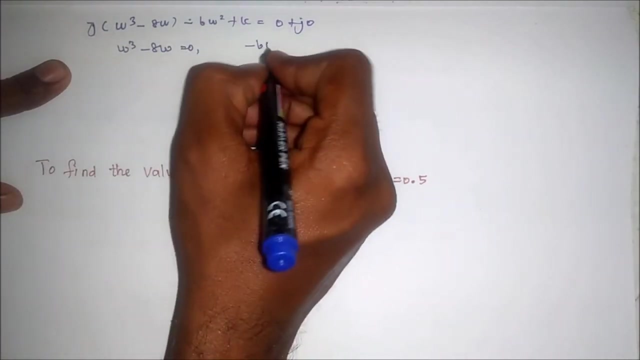 So now we can say: This is a imaginary part, This is a real part. So now, imaginary part equal to 0.. Therefore, omega cube minus 8, omega, equal to 0.. Real part minus 6 omega square plus k, equal to here, 0.. 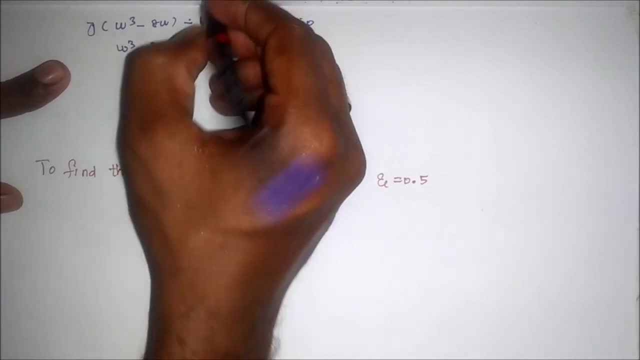 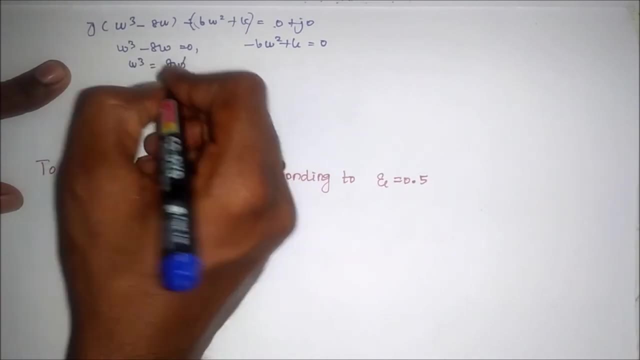 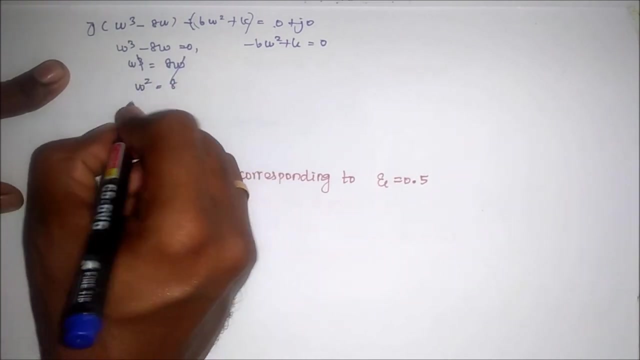 So we have to equate imaginary part and real part, both the sides. So now, This omega cube equal to 8 omega. This and here 1 omega will cancel. Therefore, omega square equal to 8.. Omega equal to plus or minus 2.8.. 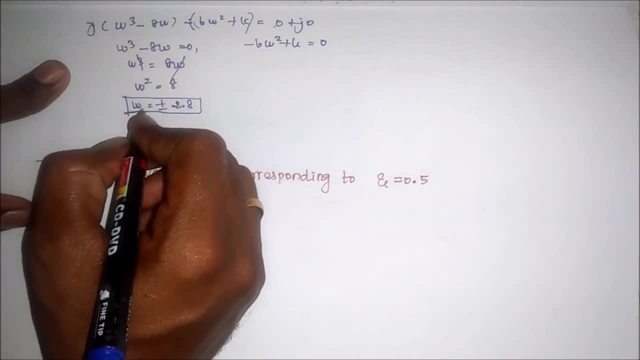 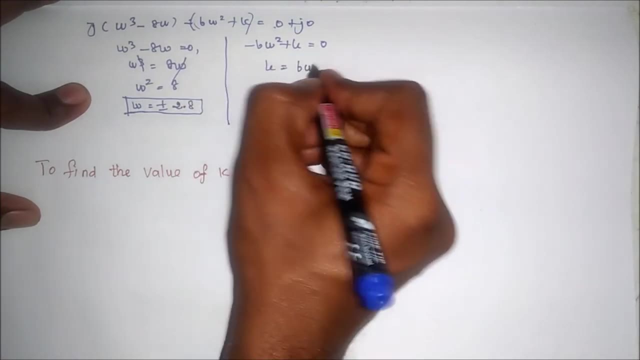 It means this is the crossing point of a root locus on the imaginary axis. Next, Gain value k equal to 6 into omega square. Here, k equal to omega square, value equal to 8.. Therefore, 6 into 8 equal to 48.. 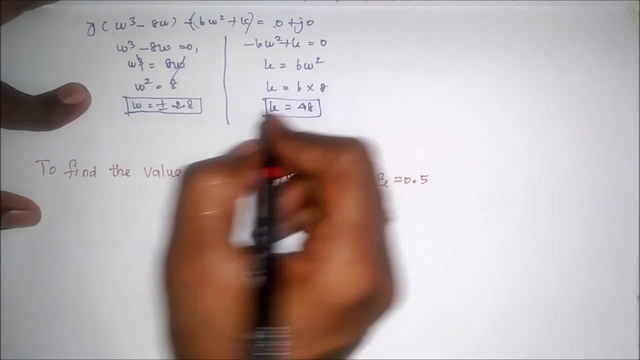 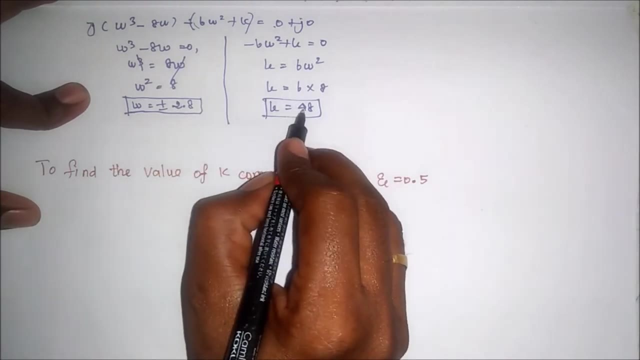 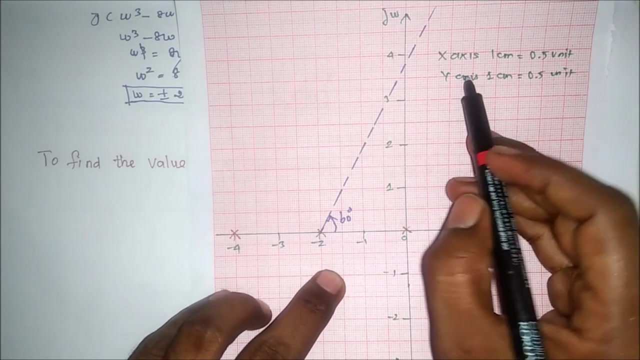 So k is the corresponding gain. We see omega is the crossing point of root locus on the imaginary axis. Its corresponding gain is 48.. So now we can construct the root locus in the graph. So we have to consider x-axis: 1 centimeter equal to 0.5 unit. 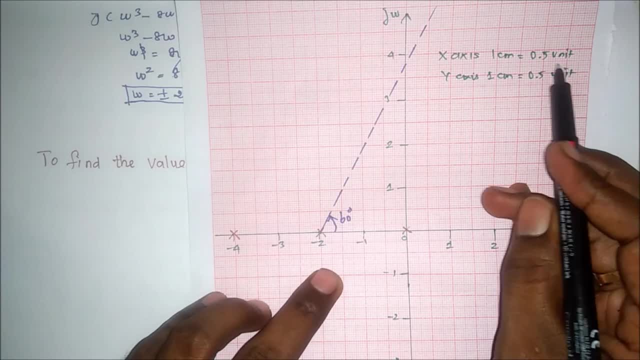 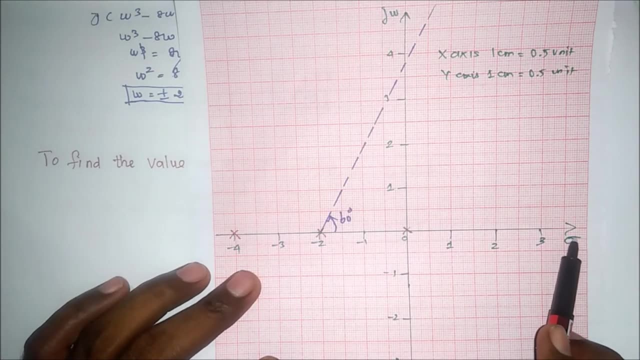 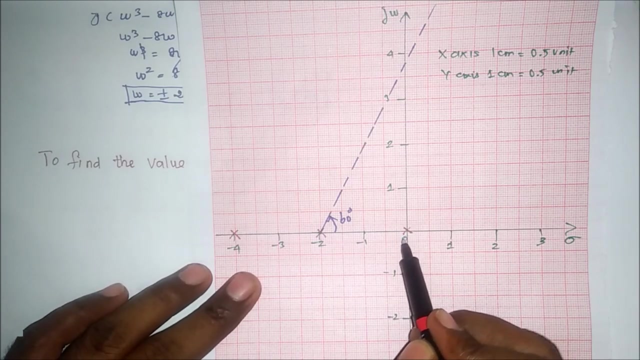 y-axis: 1 centimeter, equal to 0.5 unit. So now, after marking the axis parameters. So this is imaginary axis, This is real axis. It means x-axis. This is y-axis. So now we have to mark the number of poles by using cross mark. 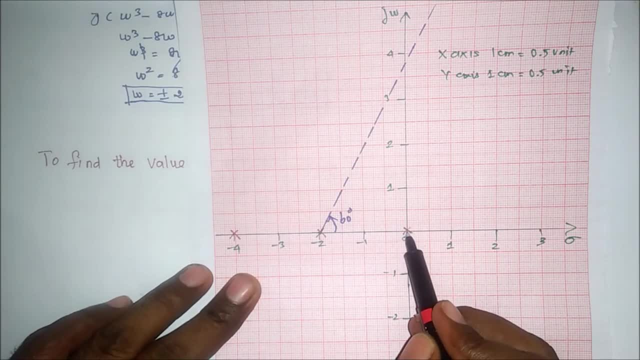 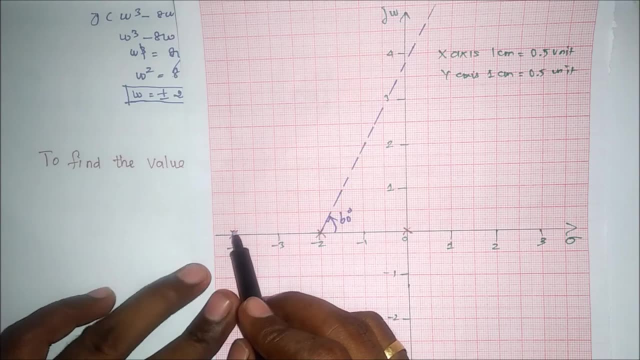 So we know here there are three poles. So pole 1 is equal to 0.. Pole 2 is equal to minus 2.. Pole 3 is equal to minus 4.. So we have to mark by using x symbol or cross mark symbol. 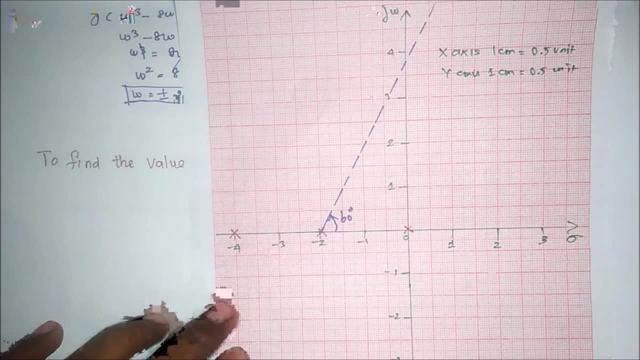 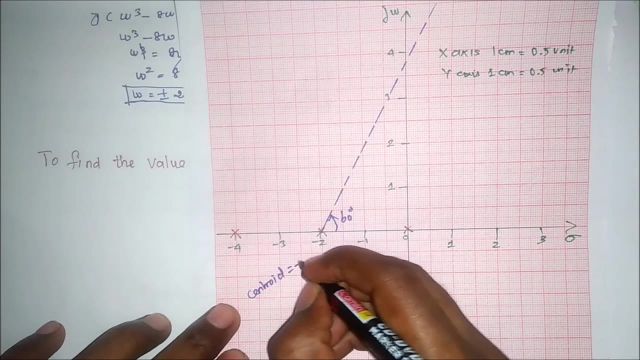 So after that. So we have to mark the centroid. So we know centroid is centroid, value equal to Centroid, value equal to Centroid, equal to minus 2.. We already calculated. So this is the centroid. So from the centroid: 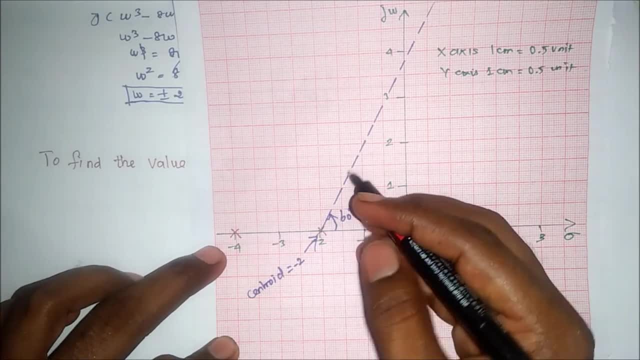 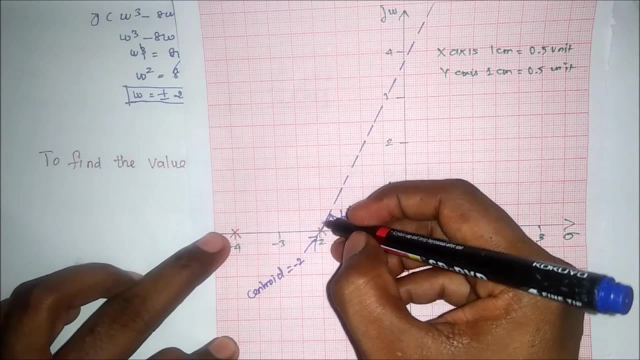 We have to take 60 degree, Then we have to draw the asymptote. So now, from the real axis, We have to mark 60 degree angle, Then we have to exactly draw a straight line with 60 degree. So this is asymptote. 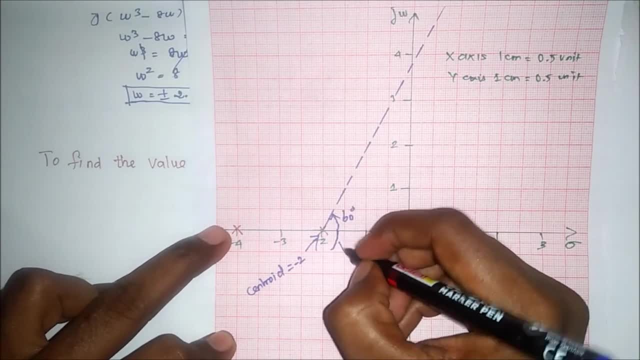 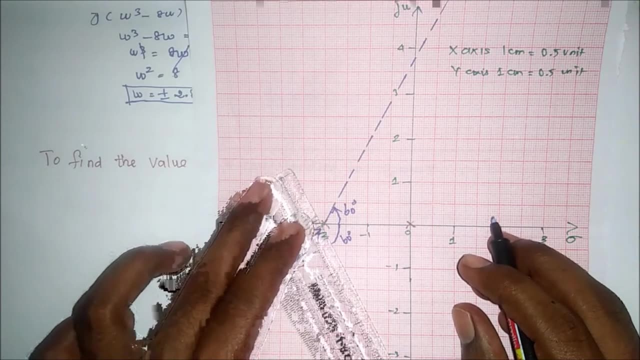 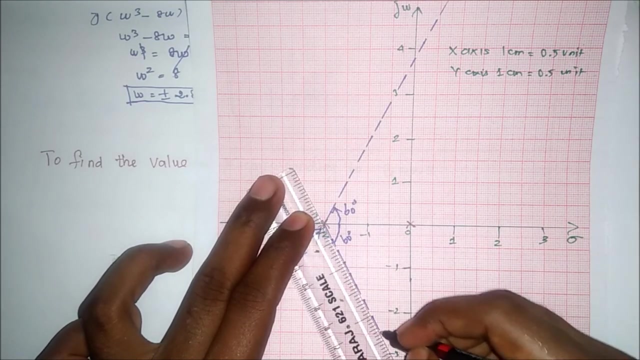 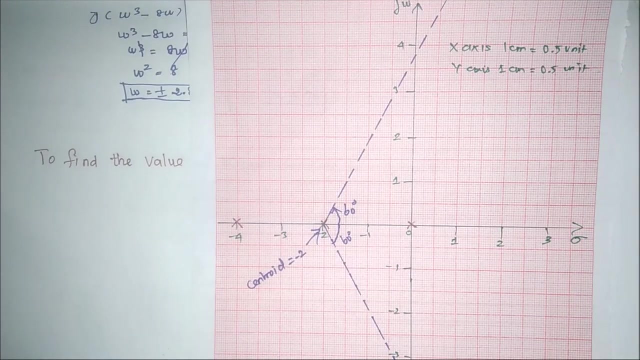 Similarly, in the bottom side also, We have to mark 60 degree with real axis, Then we have to draw the asymptote. So this is the asymptote. So after this, So here, So we know already. 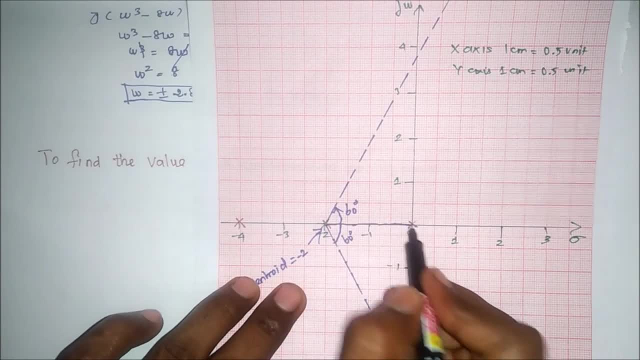 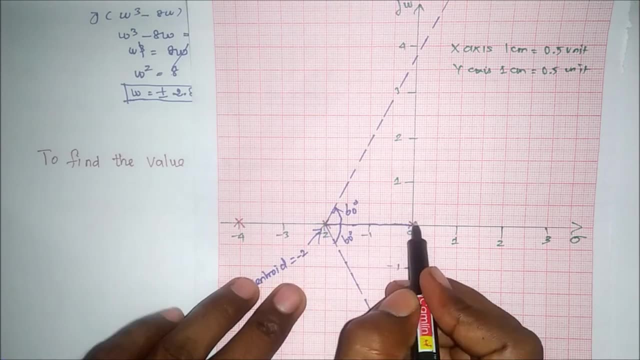 So this is a root locus. We have taken a test point at this point, After this point. So if we take a test point, between these two poles- Definitely right side- there is a odd number of poles. It means only one pole. 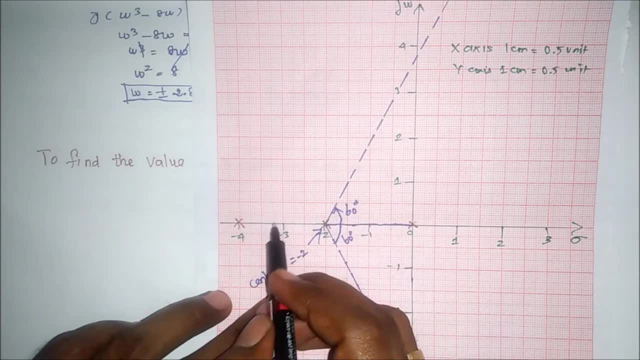 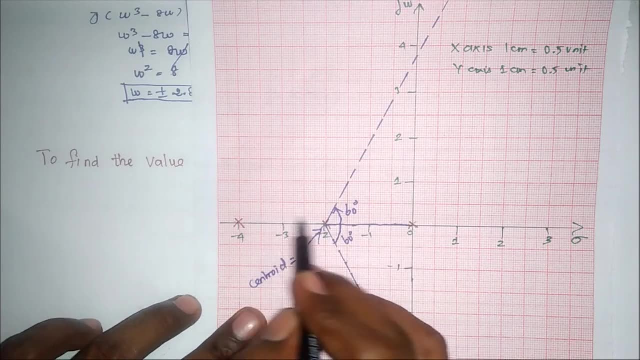 Therefore it is a part of root locus. Then if we take a test point between these two poles, Definitely in the right side of the test point There are even number of poles. Therefore it is not a part of root locus. But if we take a test point beyond this pole, up to infinity, 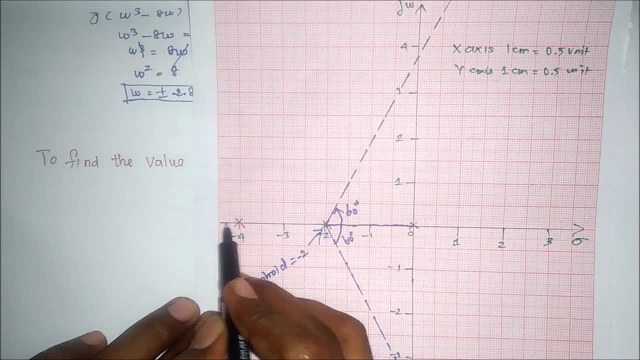 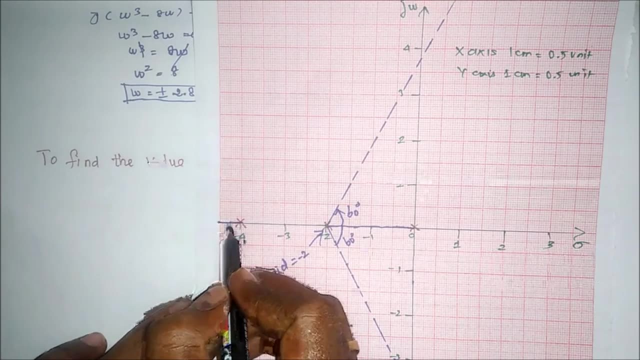 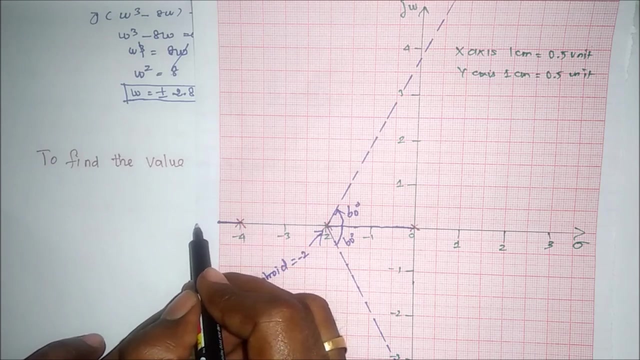 Definitely, Definitely, right hand side of the test pole will be having. There are odd number of poles. Therefore, from this point to infinity line, There is a root locus. It means this point to infinity, The negative real axis, is a part of a root locus. 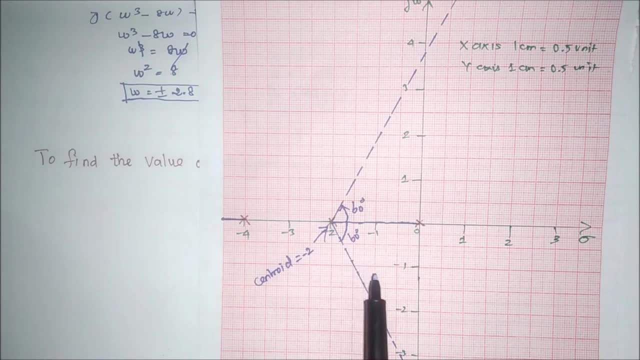 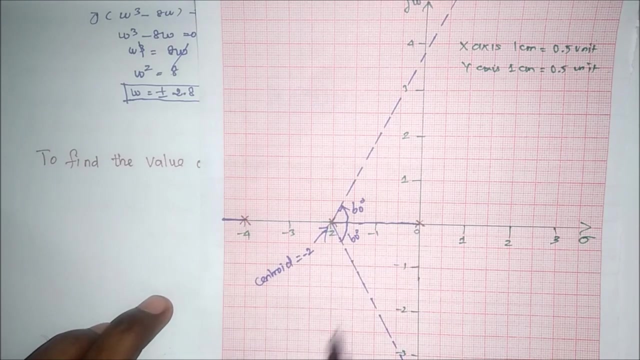 But according to the given open loop transfer function, There are three poles are available. Therefore, finally, in the root locus It will be having three number of root locus. So here, this is a root locus, This is another root locus, So we have to mark the third root locus also. 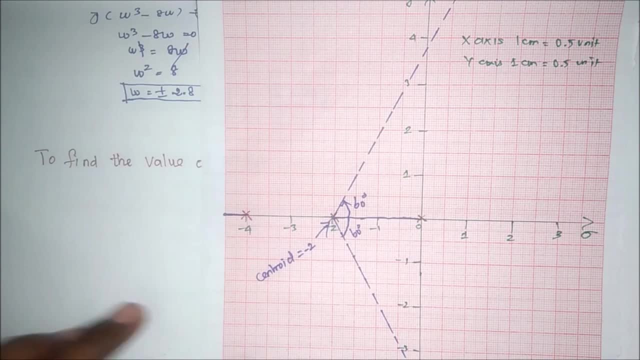 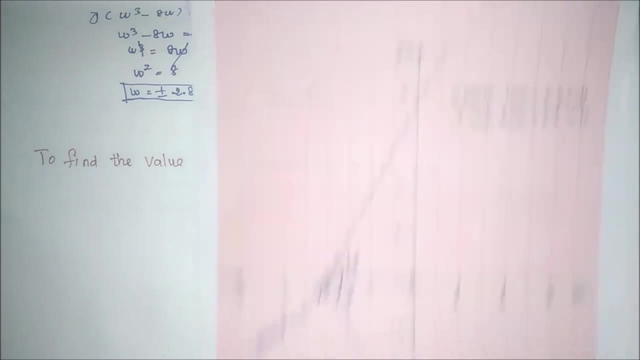 So here, in this problem, We found there is no angle of departure. Therefore we have to consider the. So we have to consider the breakaway points Minus 0.845.. Therefore, in this negative real axis, We have to mark the 0.854.. 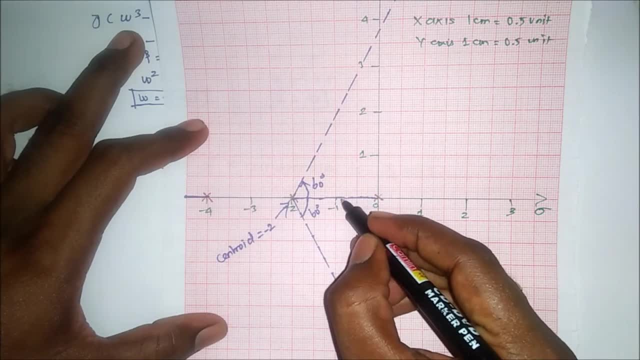 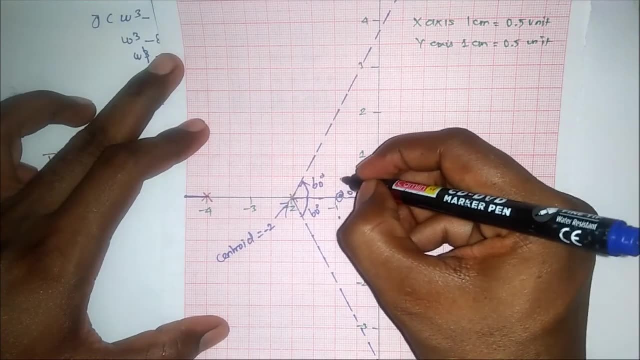 So actually this is 1.. This is 0.5.. So it will be 0.854.. So this is 0.854.. So definitely. So we have to draw small straight line, So a root locus. 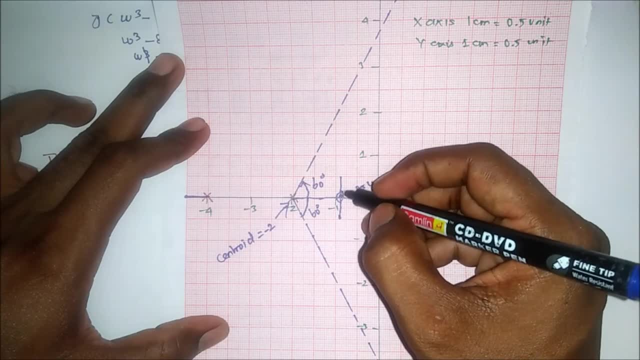 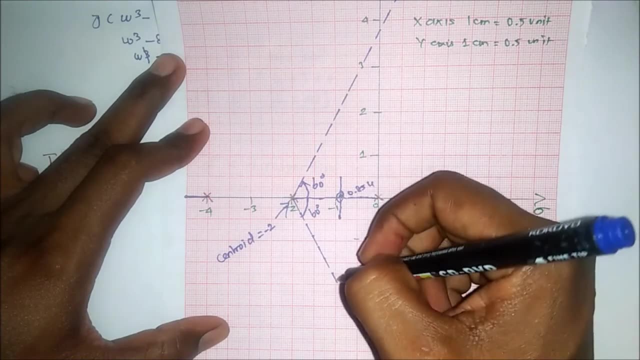 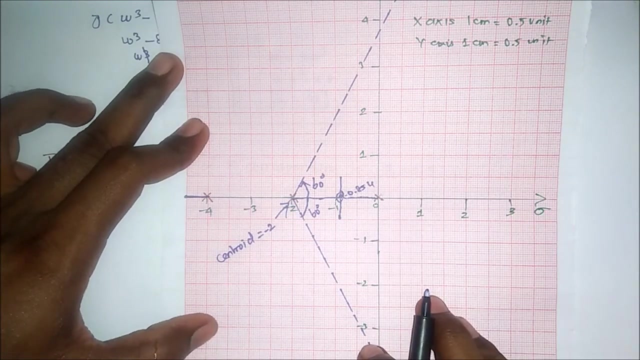 It means third root locus Will cross- break away at this point. So there will be a root locus That is parallel with this asymptote, That will break away at this point, So it will be 0.854.. Therefore. 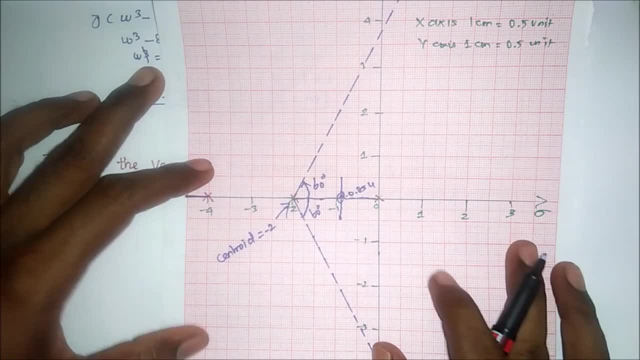 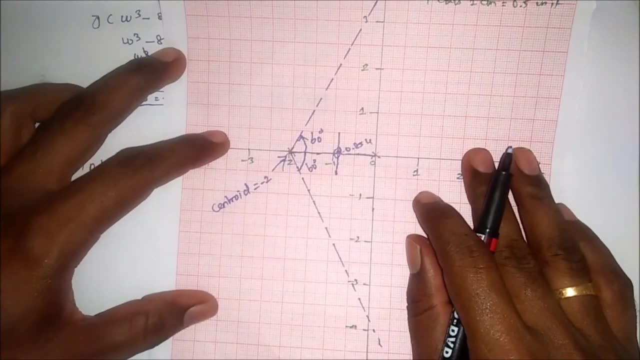 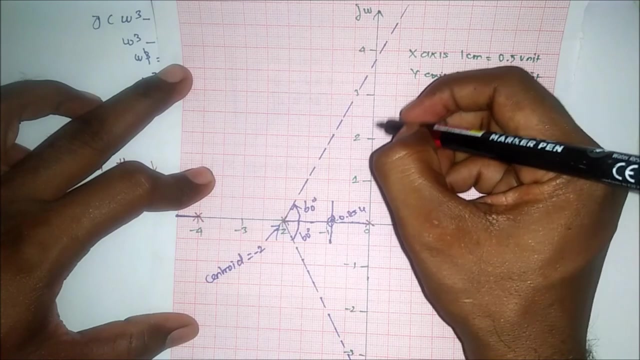 So we already calculated the crossing points. So crossing point equal to Omega, equal to plus or minus 2.8.. Therefore, in this imaginary axis We have to mark Plus 2.8.. So this is 2.5.. 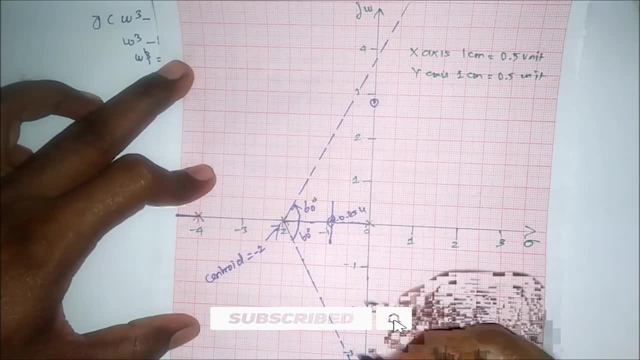 So this will be the 2.8.. In the negative side also, We have to mark 2.8.. So this will be the 2.8.. So this will be the 2.8.. So now we have to connect. 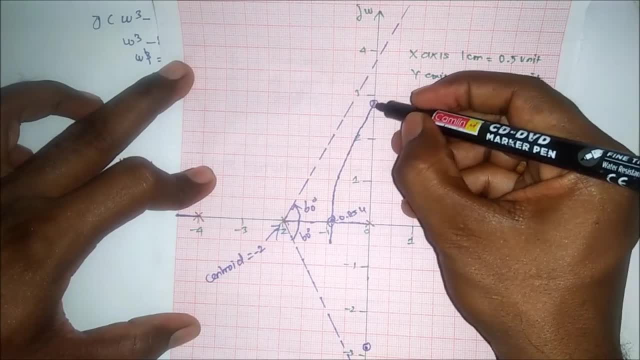 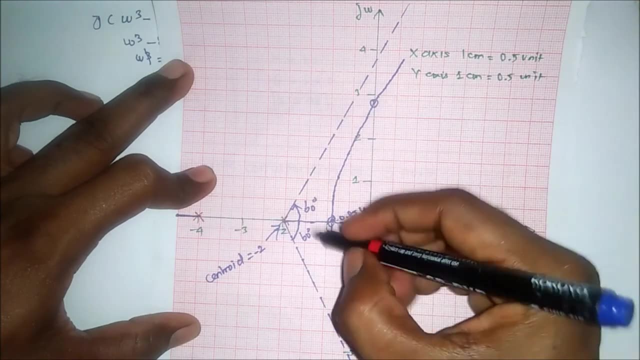 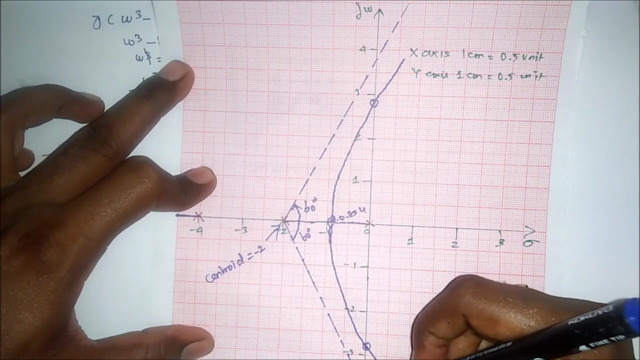 So now This root locus will Move parallel with this asymptote. It will go up to infinity. So here also It will cross at this point. This will go parallel with this asymptote, Then it will go up to infinity. 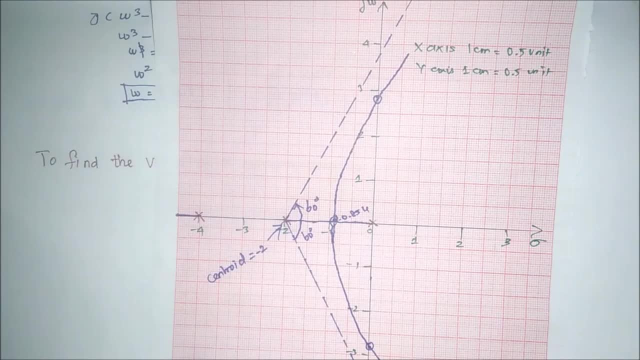 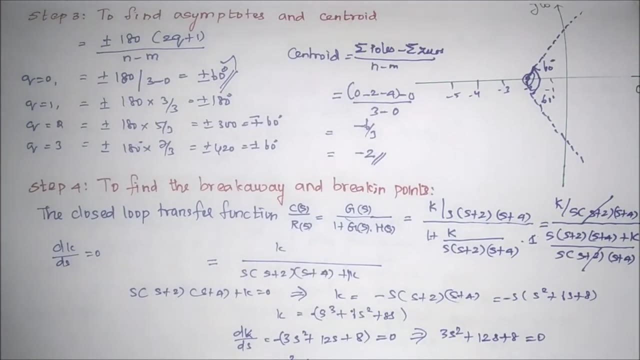 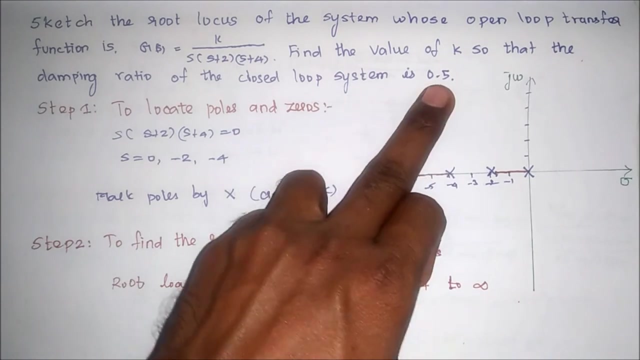 So now this is the final root locus, But according to the given problem. So actually the given problem says that Find the value of k, So that the damping ratio of The transfer function is 0.5.. So now, 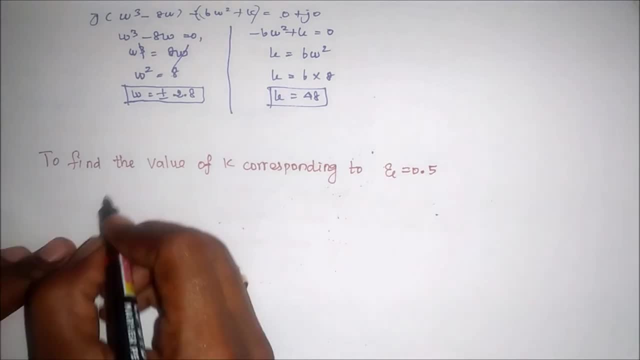 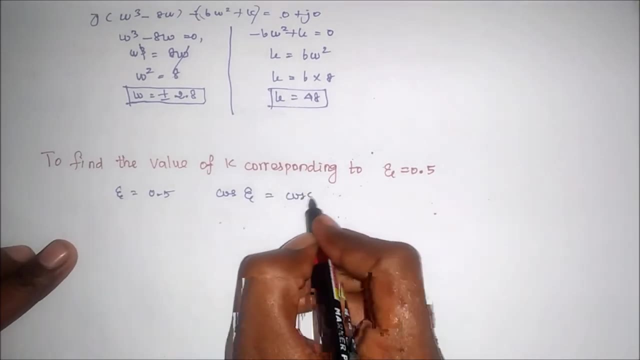 Damping value is nothing but eta. So we know Eta equal to 0.5.. Therefore, Cos eta equal to Cos 0.5, equal to 60 degree. So what we have to do? So in this, 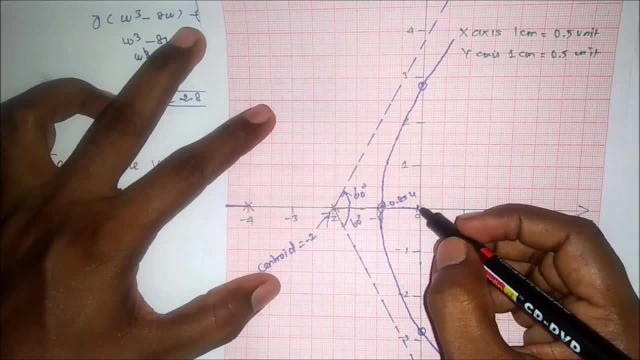 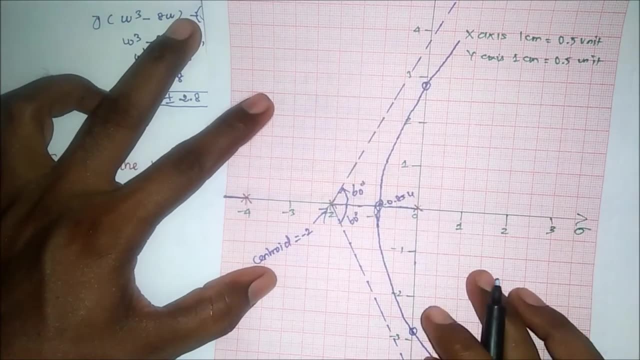 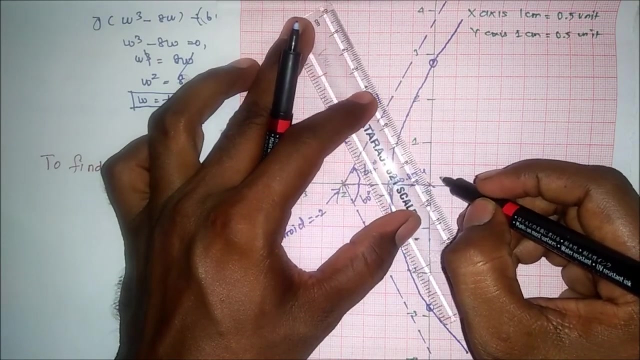 From this point. So we have to take 60 degree, We have to take 60 degree from the real axis, Then we have to draw a straight line. So if we draw, Actually, According to the eta Cos, theta value equal to: 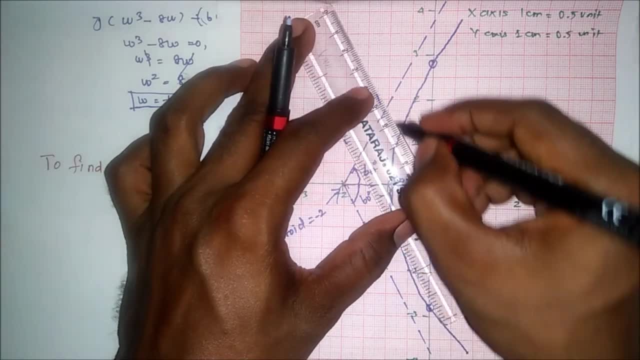 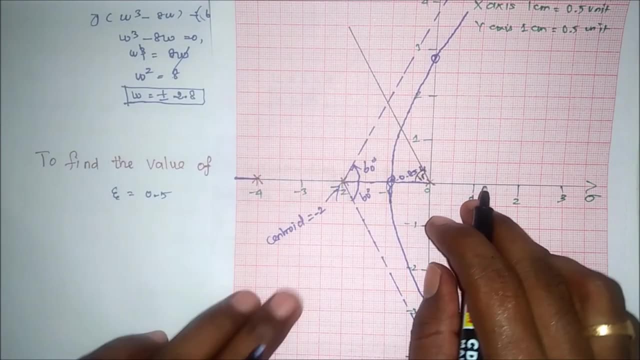 60 degree Therefore. So we have to draw a 60 degree line, So this is 60 degree. So now, So it will touch a point In the root locus. From this We have to mark a. 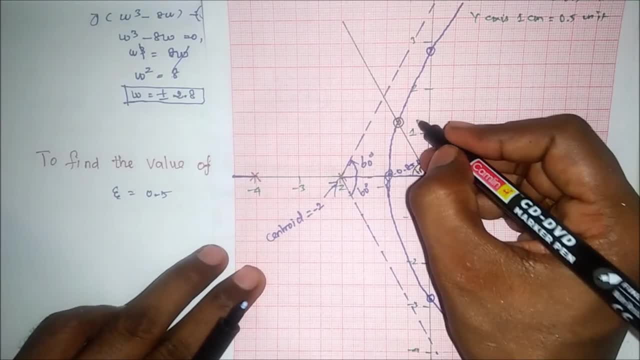 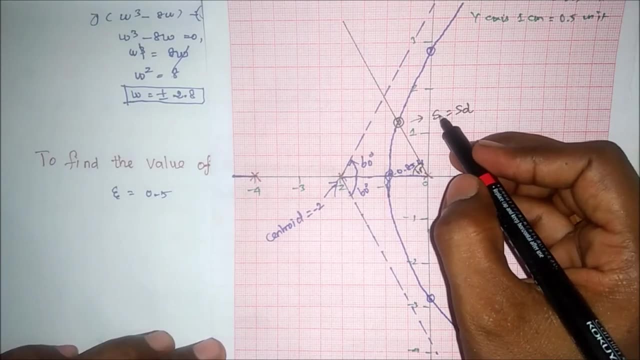 So now This we can say: It is a Dominant pole s equal to sd. So from this Dominant pole, So we have to connect all the Existing poles. So now We have to connect the. 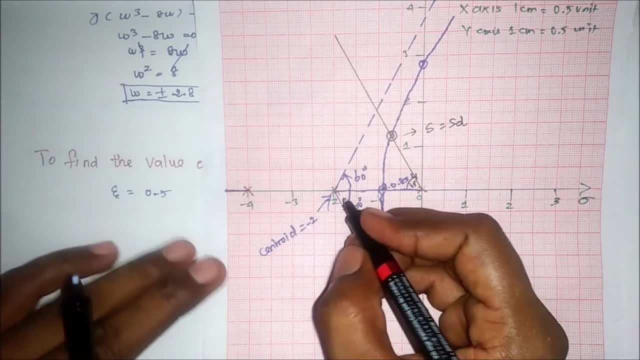 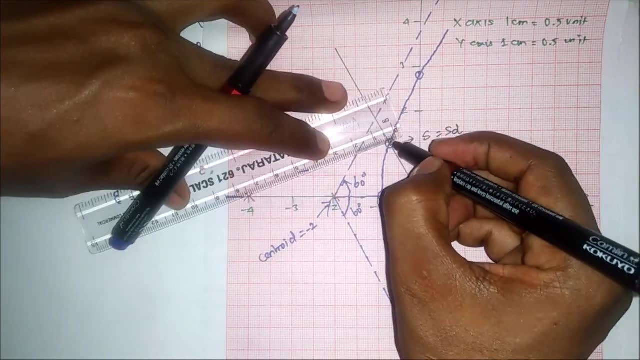 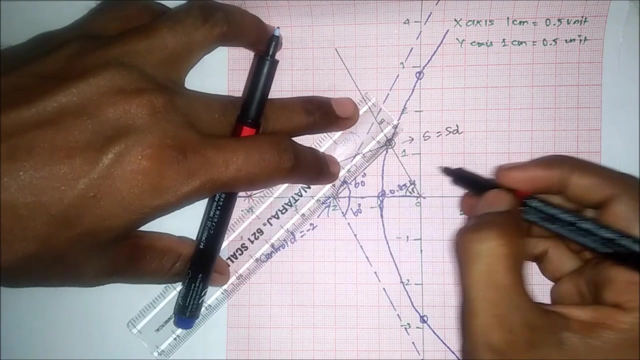 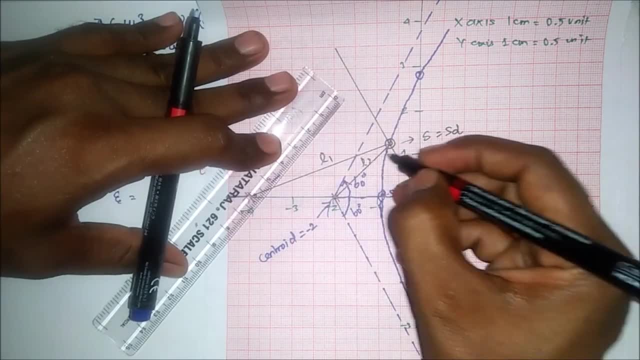 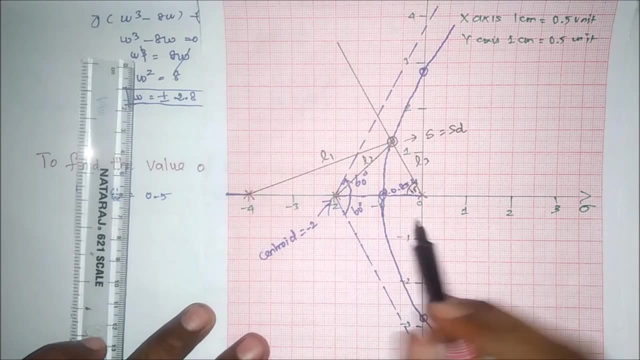 Already. This is connected, So we can say It is a Length 1.. This is Length 2.. This is Length 3.. So now We have to find the value of L1., L2.. 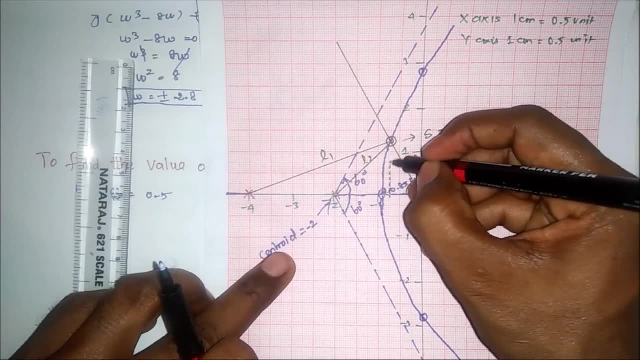 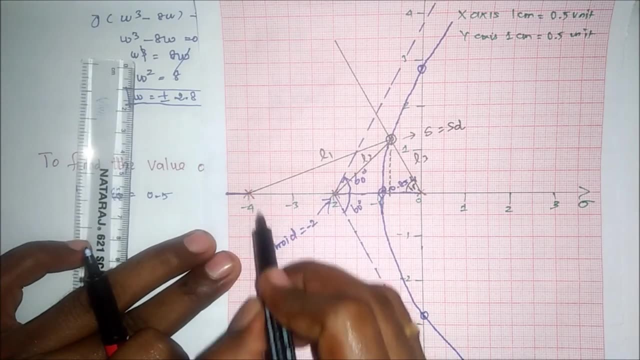 L3.. So now, So we can Mark this point, This point, So now We see It is. So this part is A Right angle Triangle. We can say A, A Equal to. 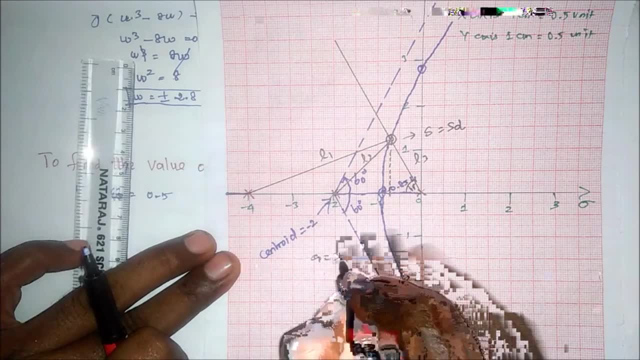 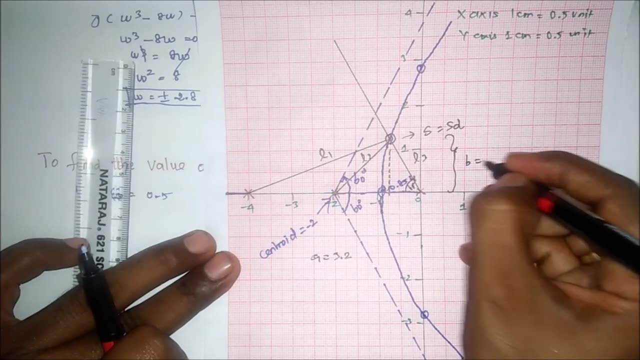 What is the value of A? 1., 2., 3.. So we can say 3., 2., The bottom, 3. 2.. Here It is. We can say B. So now. 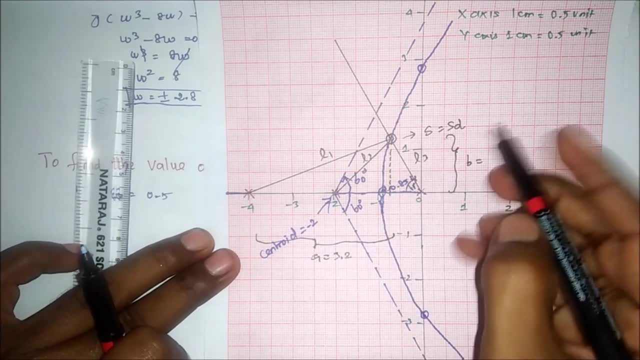 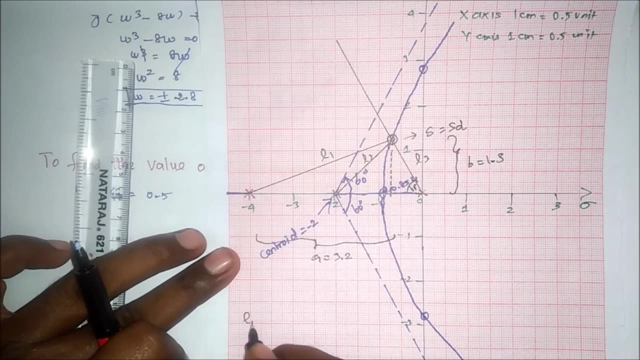 This is: We can say A From this point To this point, So B Value Equal to 0., 3.. So we can calculate The value of L1.. Next L2.. So now. 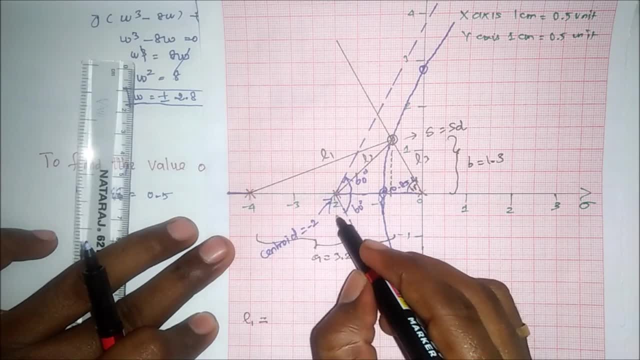 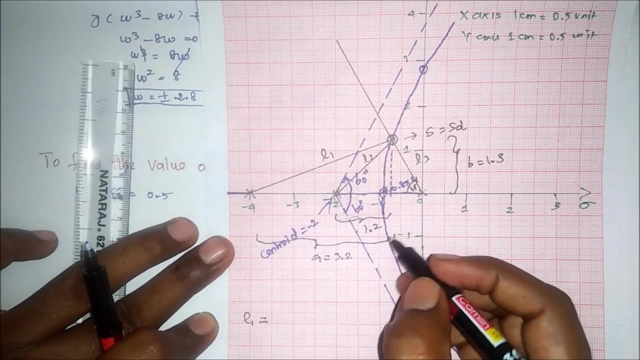 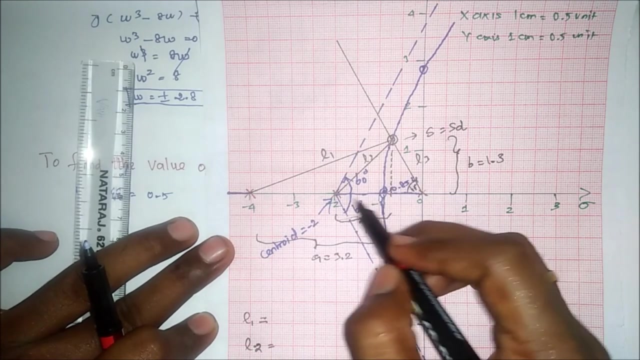 B Is 1.. 3. Same, But We can consider This As A Right angle Triangle, So now Its Value Equal to This Is 1.. This Is 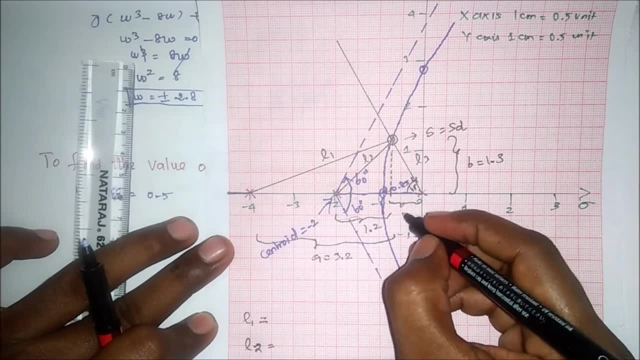 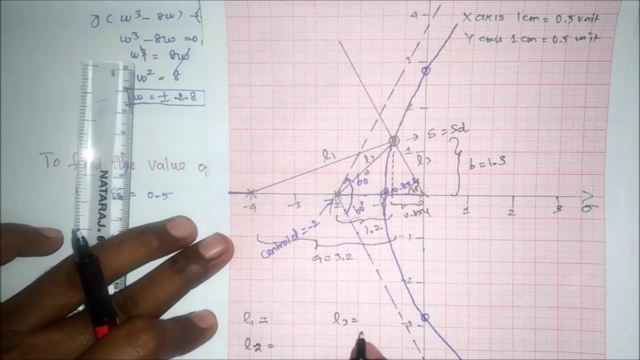 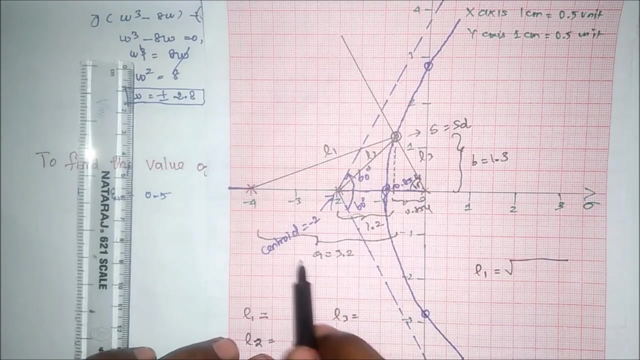 2. So now, With This Value Is 0.854.. 0.3.. So now, By Using Pythagoras Theorem, We Can Calculate The Value Of. 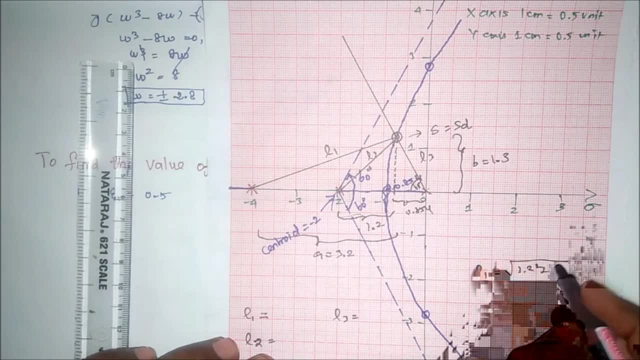 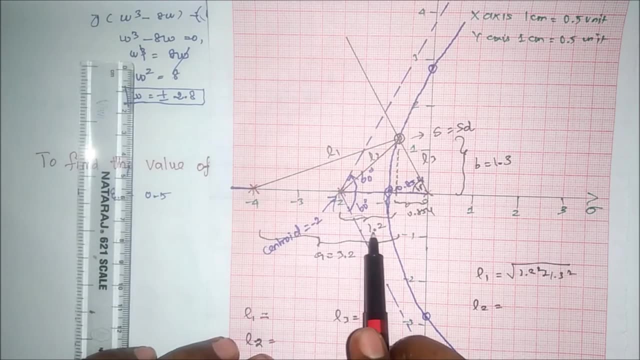 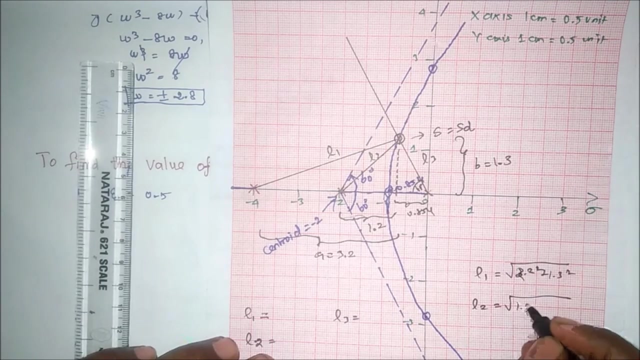 L1.. It Means So now L1.. Equal to Square Root Of Adjacent Side 3.. This One Square Root Of, So this Is 3.2.. 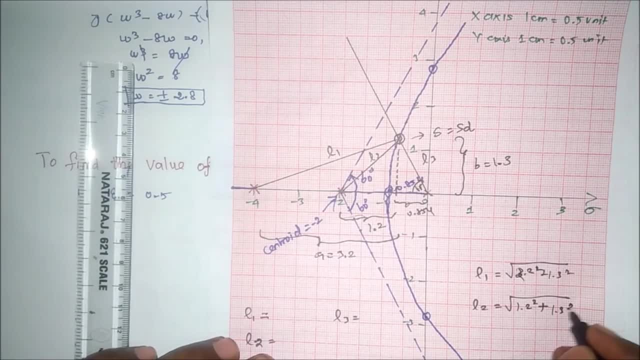 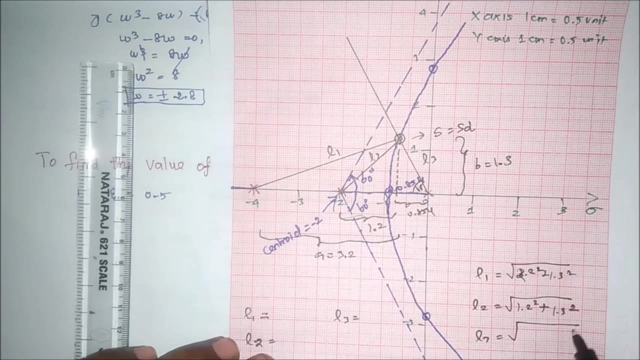 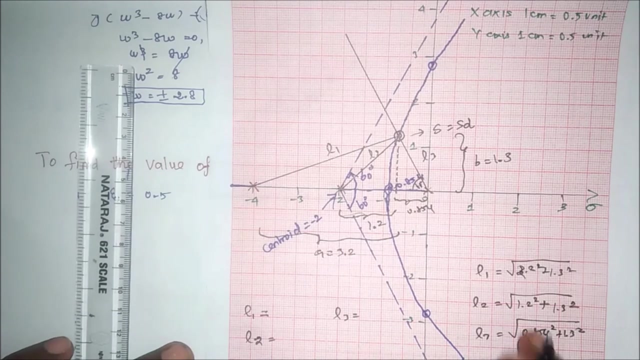 1. 2. Square Plus Its Opposite Side Value Equal to 1. 3. So now L3. Equal to For This Right Angle Triangle, Opposite. 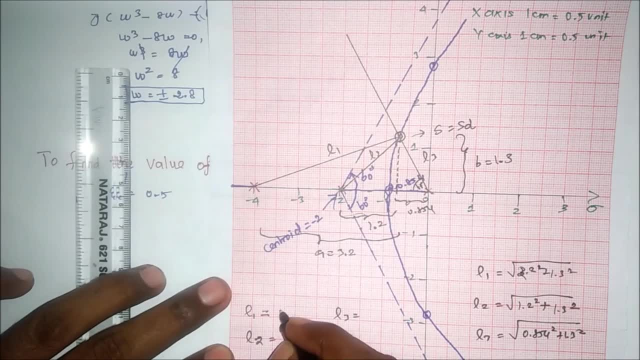 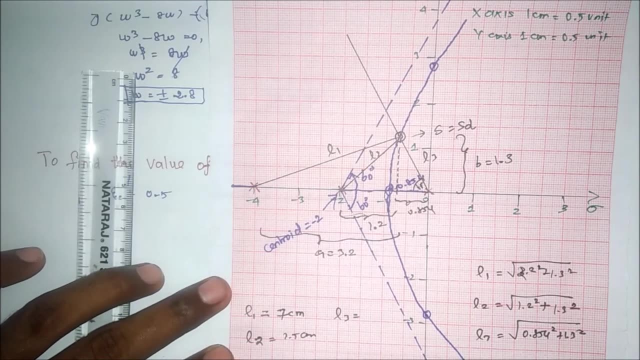 Side: L1. Equal to 7. Centimetre. L2. Equal to 3.5. Centimetre. L3. Equal to 2.5. Centimetre. So now We: 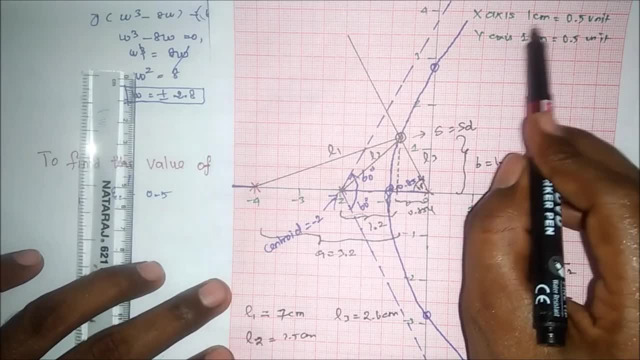 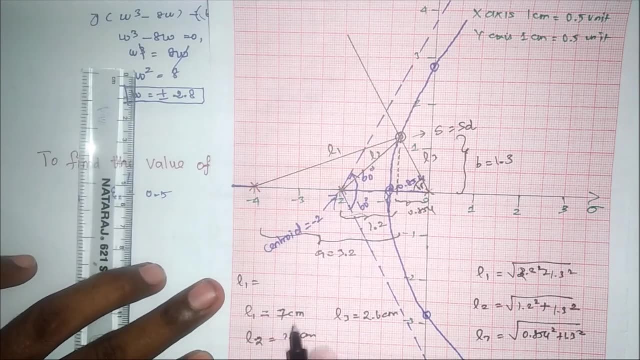 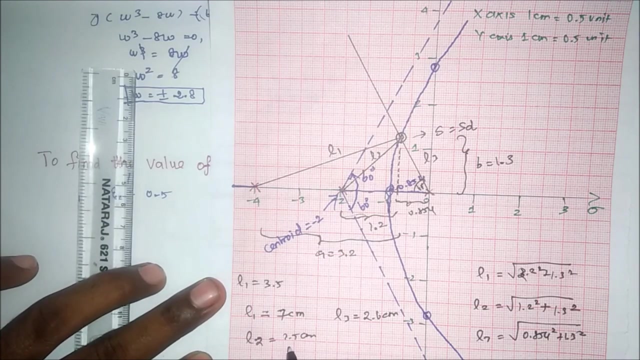 Know From The Axis 1. Centimetre Equal to 0.5.. Unit. Therefore, Finally, We Can Write L1.. Equal to 3.5.. Into 0.5.. 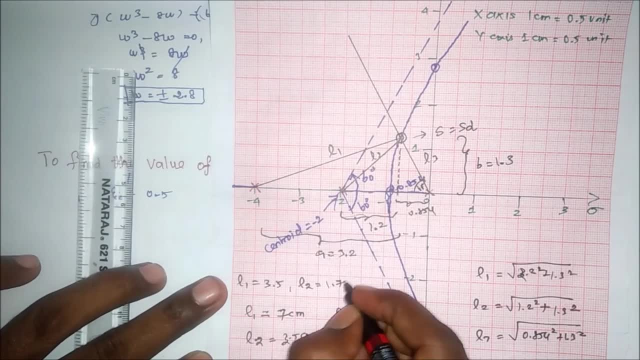 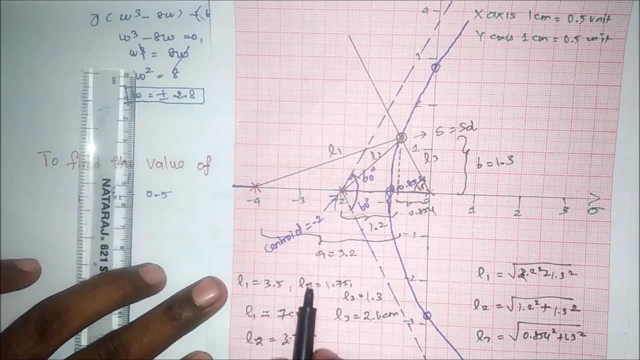 3.5.. Into 0.5.. Equal to 1.75.. L3.. Equal to 2.6.. Into 0.5.. 1.3.. So now This Is. 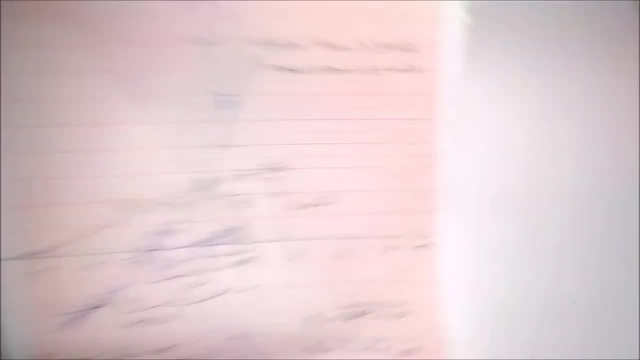 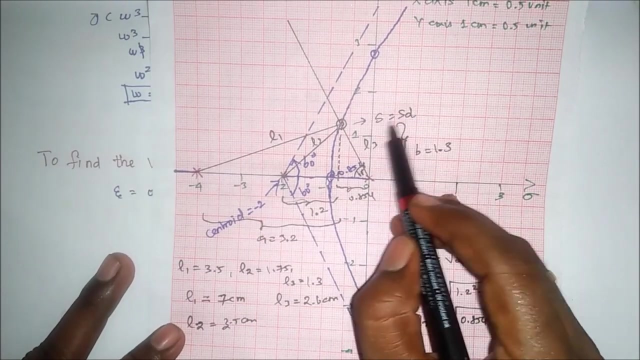 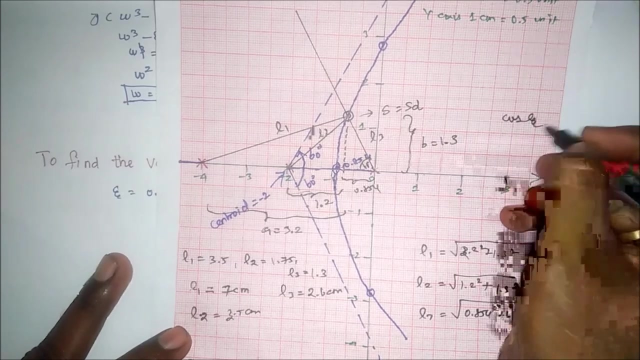 The L1. Value, L2. Value, L3. Value, So from This Dominant Fold. Actually, How We Calculated This Dominant Fold, The Given Eta?